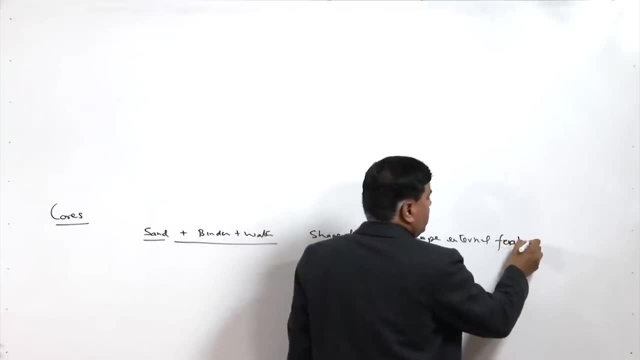 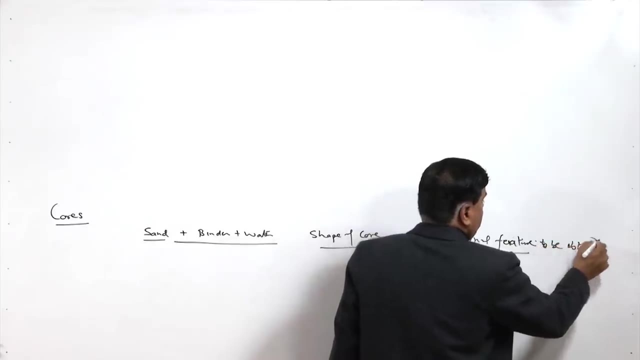 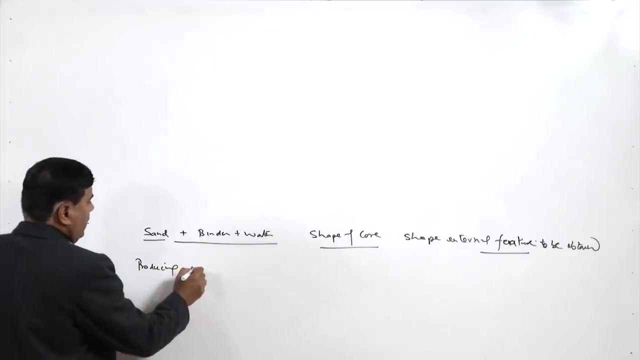 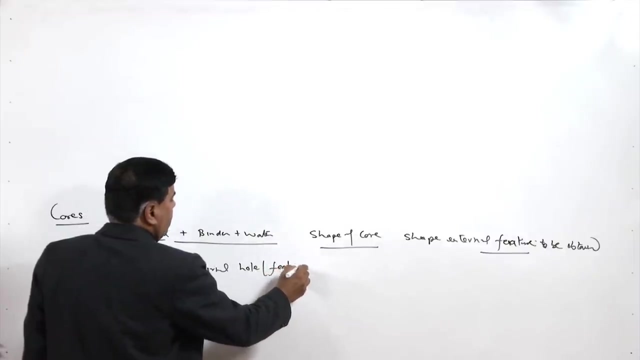 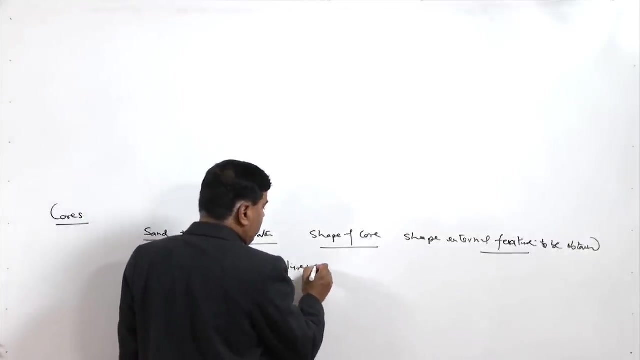 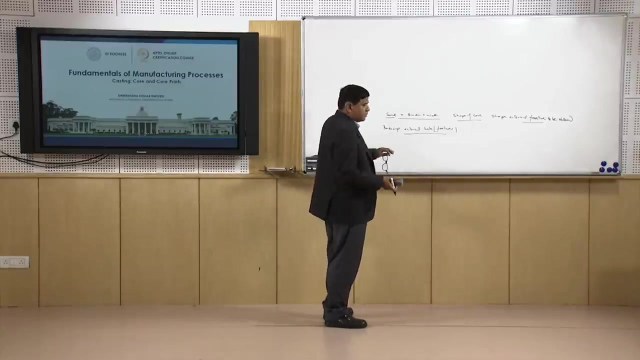 is the core print. So basically, cores are used for producing the internal holes and features which otherwise cannot be produced in the mould with the help of the patterns. So those features which cannot be produced using the pattern into the mould, and so the castings cannot be produced of the desired size and shape with the internal features. 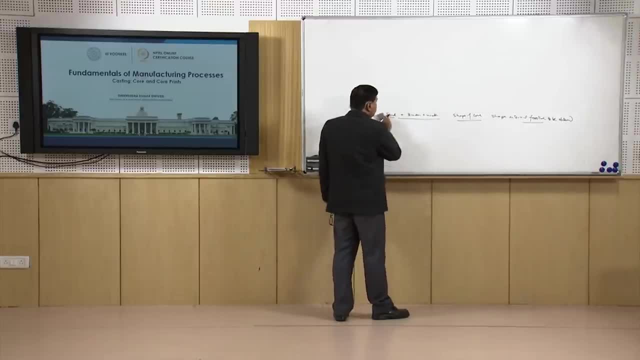 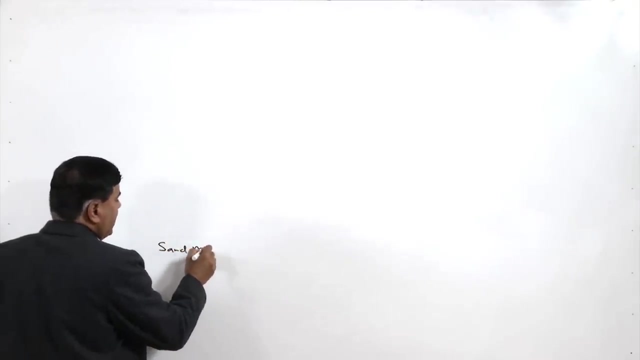 So for those situations cores are used. So basically, the cores core is located in the mould, in at the location desired so that the internal feature and the cavity can be created. So the cores are not used. means are not used only with the sand moulding For producing. 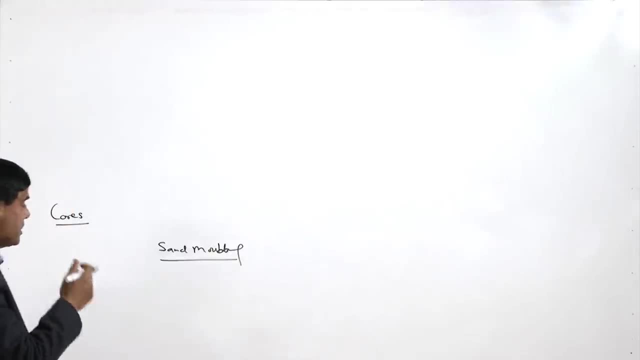 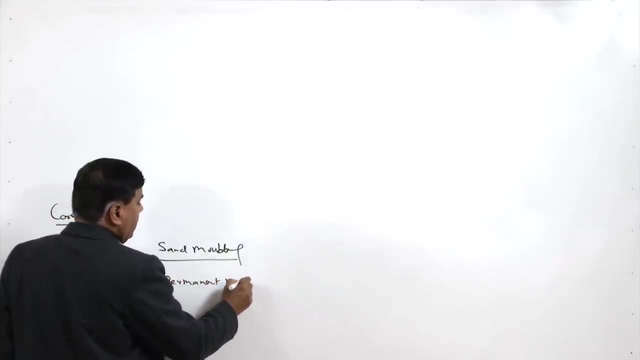 the internal features. of course the cores are used in the sand moulding, but not only the sand moulding. also in permanent moulds cores are used, So that in the permanent moulds- means these will be the made of, these are the metallic moulds- and in the metallic 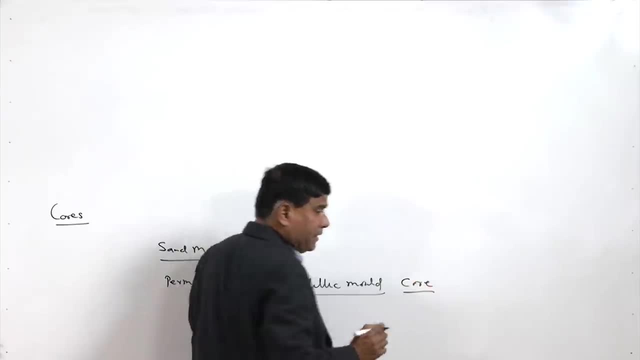 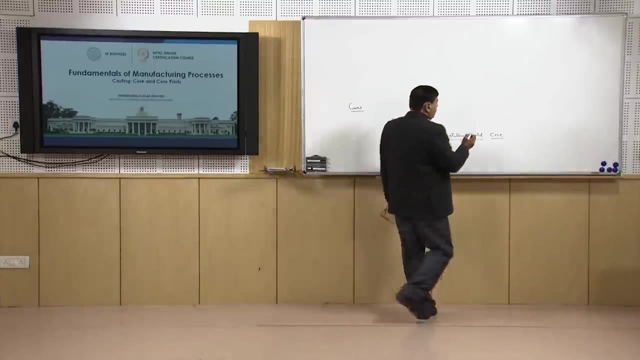 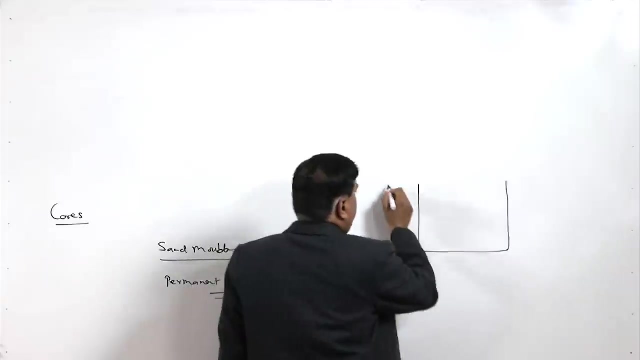 moulds, the core is positioned suitably So that internal feature and the cavity or the hole can be produced. So we will see one typical diagram like this: a simple mould like this: So this is the sand mould. So what is done to make a component with the hole like this: 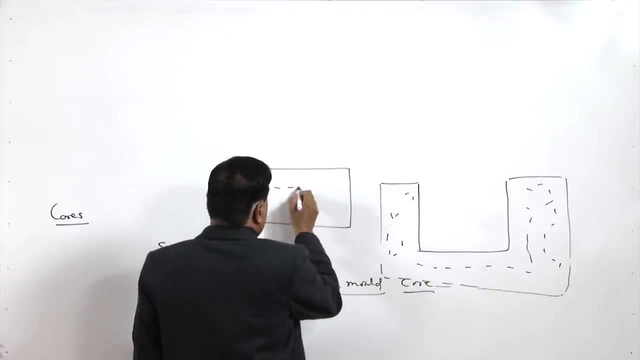 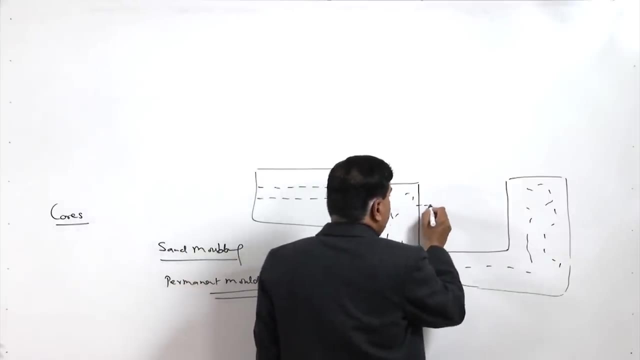 through hole like this can be produced with the help of the core. So for this purpose, we need to locate one core at this position, suitably where it was the desired. So, basically, this core made of the sand or coarse sand plus binder, plus water, and it is positioned. 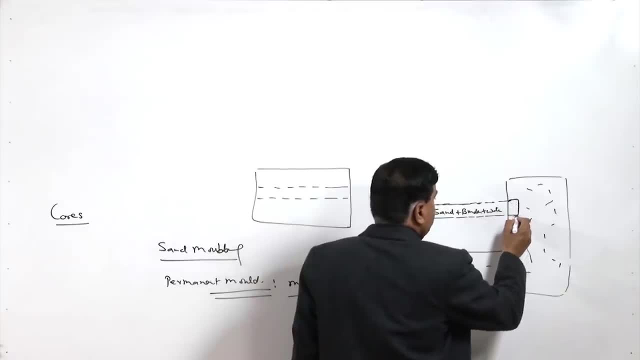 at the desired location. So this portion of the mould provides the seat for the core. 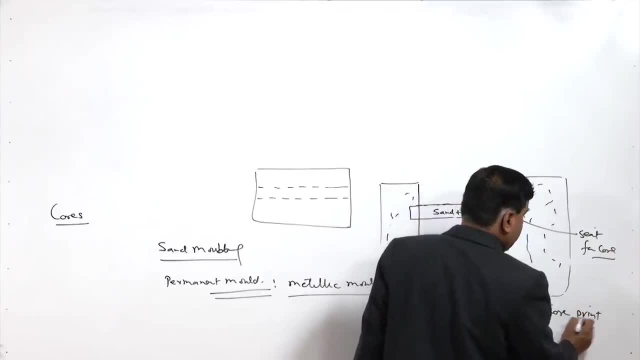 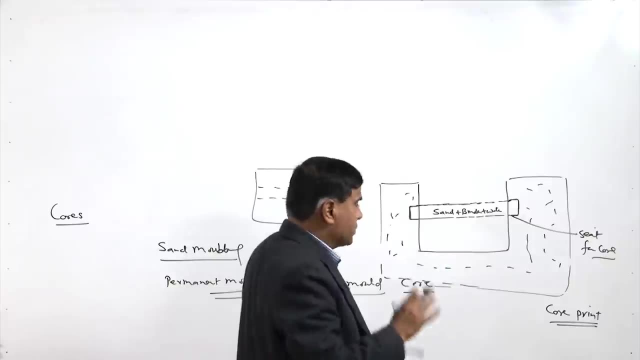 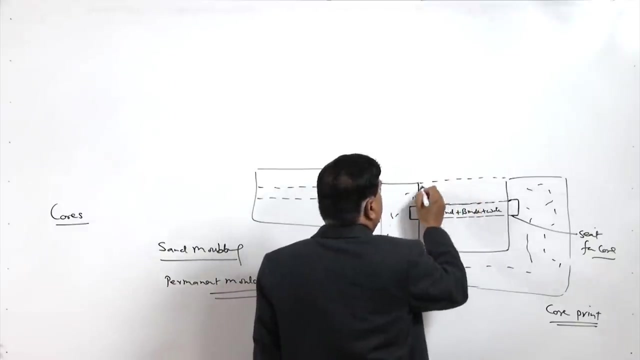 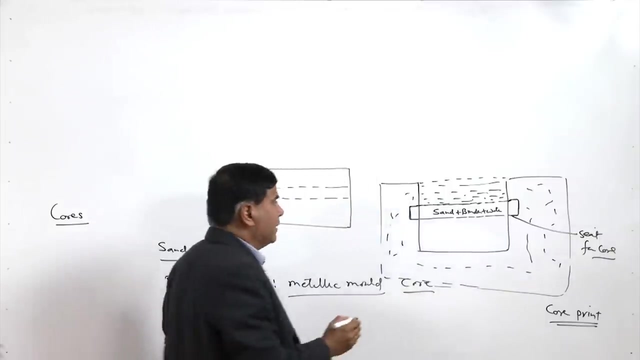 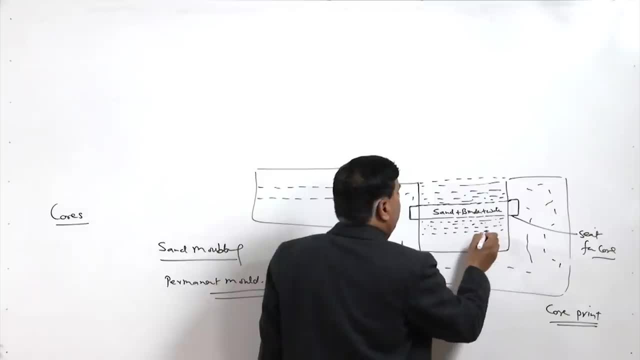 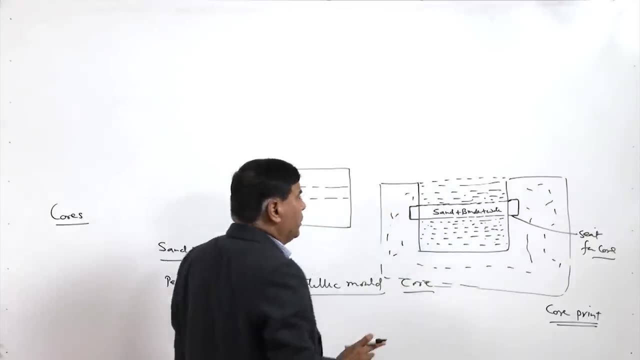 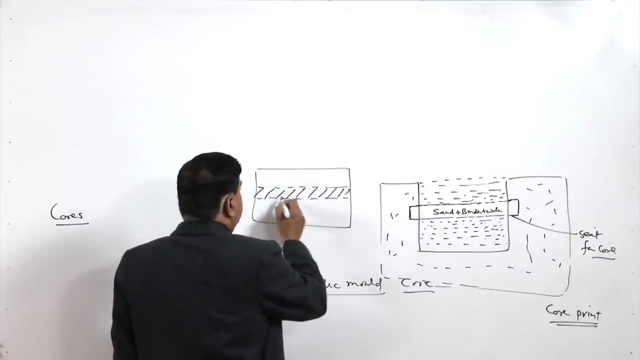 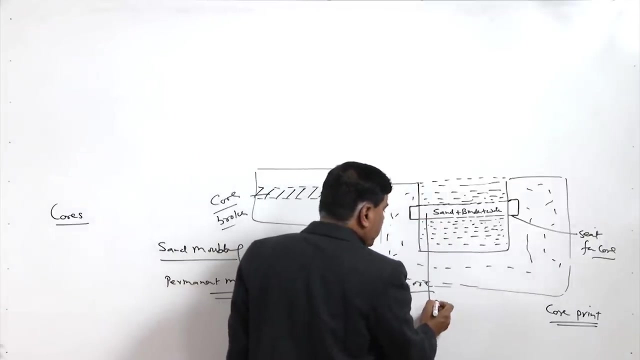 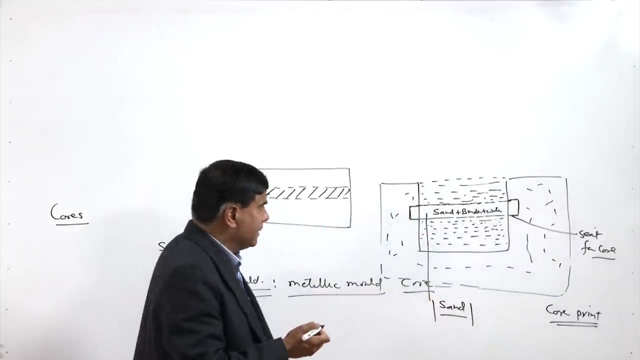 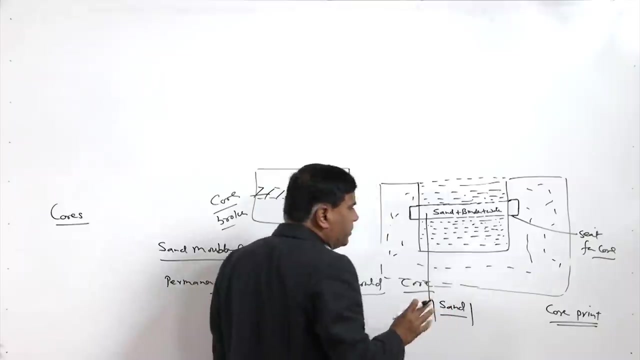 Normally the core is made of the core sand and the density is quite low of the core sand material as compared to the casting metals and that is why the forces act on to the core due to the density difference as per the volume of the metal displaced by the core. 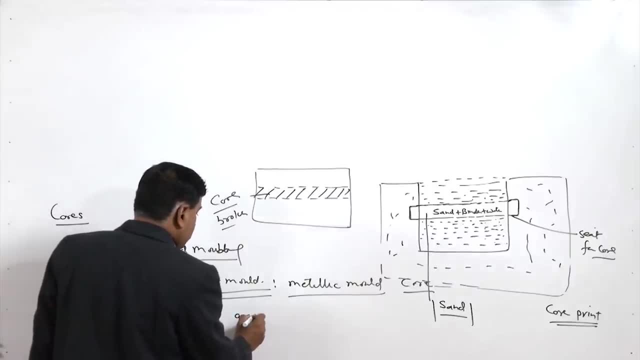 Two types of the forces are there. one is the gravitational force acting on to the core, and another is buoyancy force, or the force which is trying to lift the core in upward direction, due to the density difference, because the core is generally lighter than the metal which is used for the casting, and because of this, 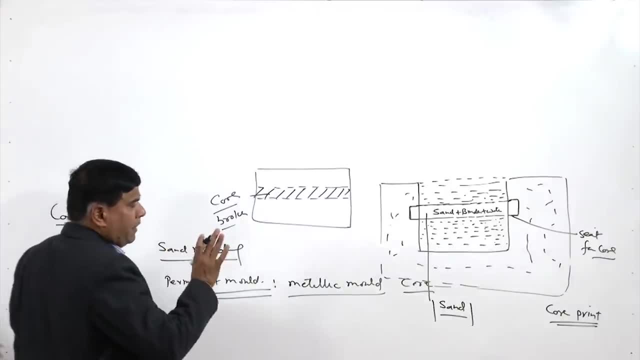 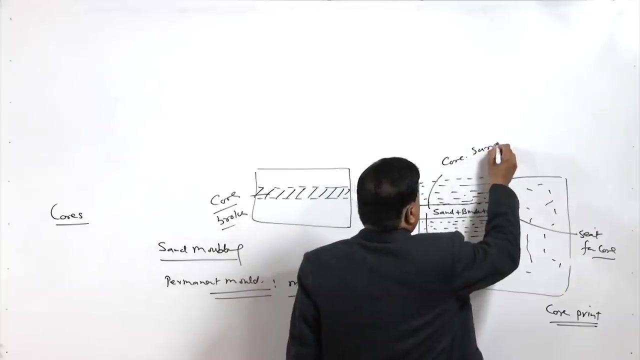 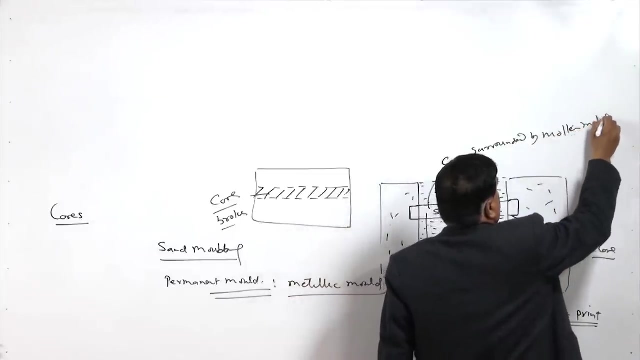 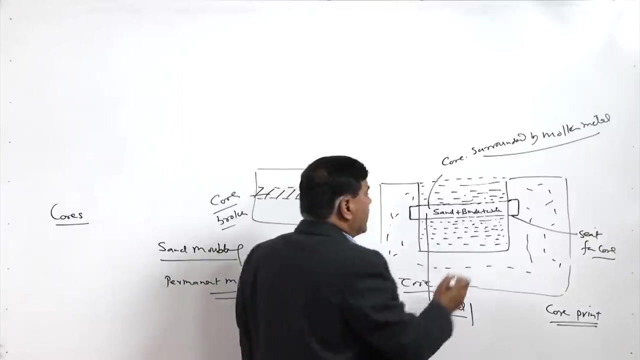 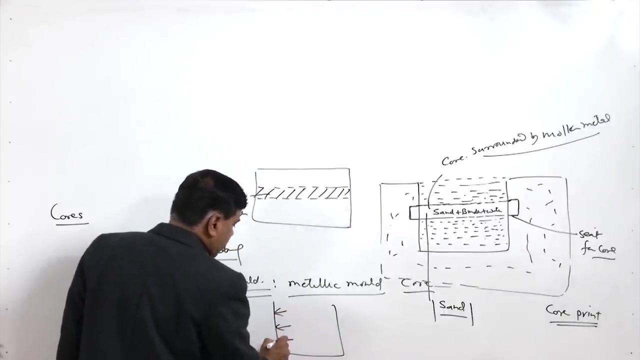 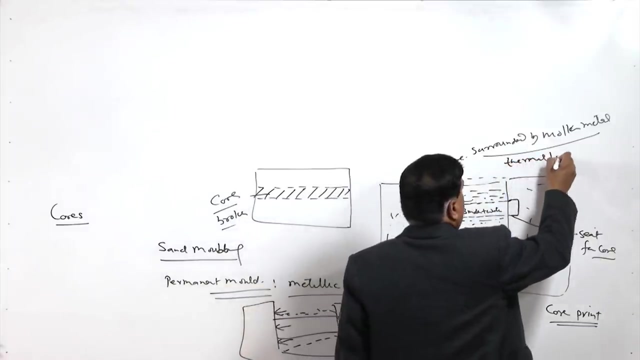 it is required that the core is able to withstand under the forces acting in presence of the molten metal. So basically, if we see this scenario, the core is surrounded by molten metal. this is one. So this is the thermal heating as compared to the mould wall. If we see the mould wall, mould wall experiences the heat means it is exposed to the molten metal from one side only, but in case of the core it is surrounded from all the sides. So the kind of heat which is experienced by the core is much severe. 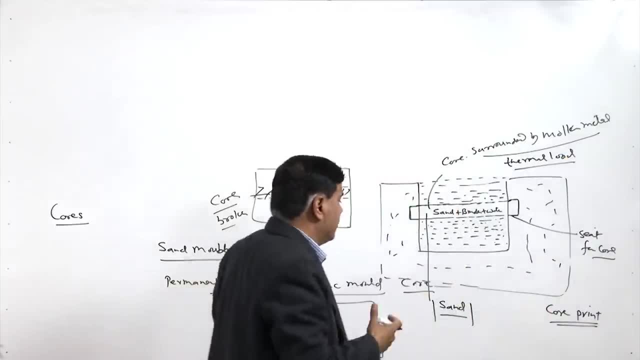 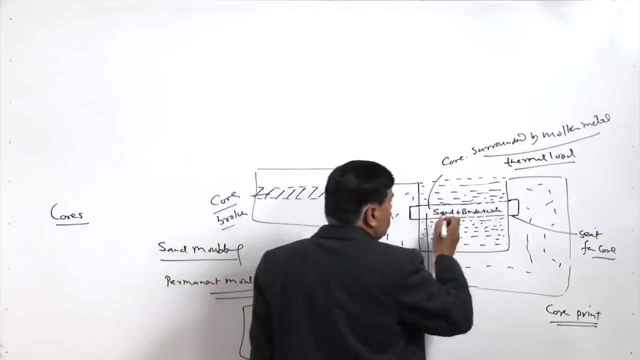 So this kind of heat on the core is much higher as compared to the mould walls. Similarly, the forces which will be acting like the matlo static pressure experienced by the core, as well as the weight of the core, well as the weight of the core, these two in combination when work together. basically, 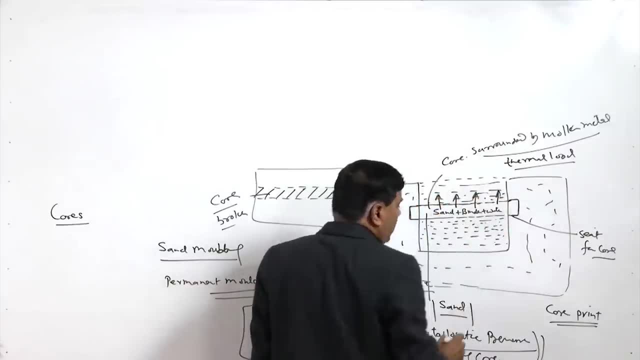 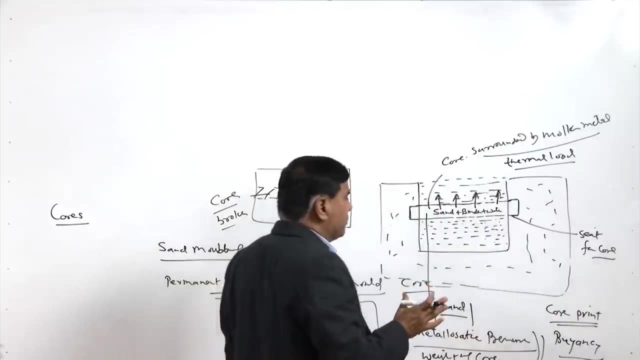 there is a lifting of force due to, or which is also called buoyancy force, which acts on to the core because of the density difference of the molten metal and the core material. So, and this is much higher than the kind of load which is experienced by the walls. 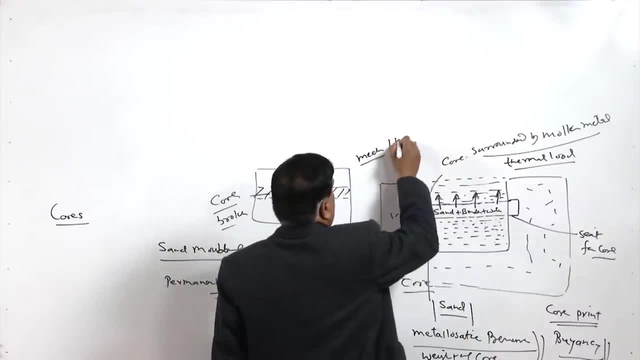 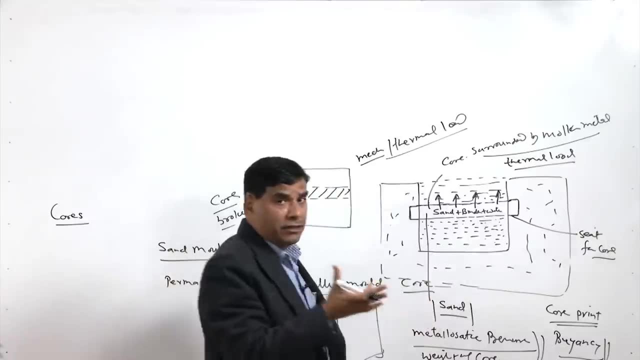 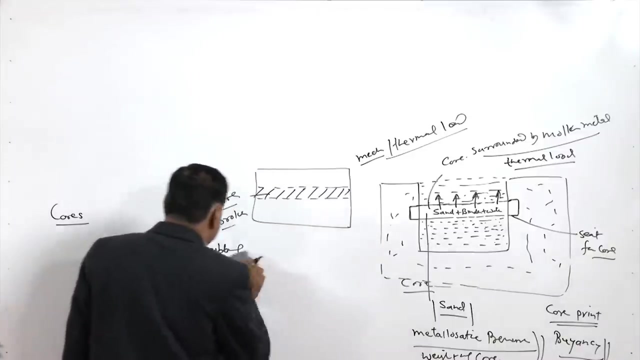 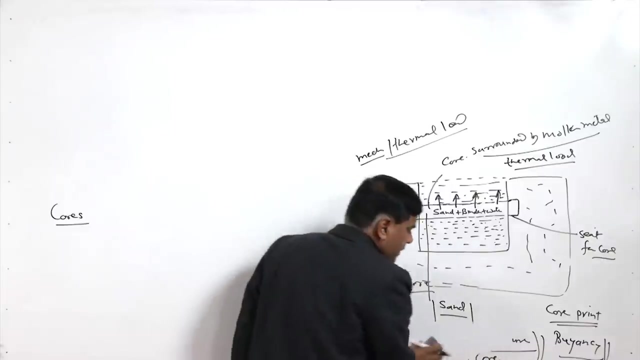 So both mechanical and the thermal load. thermal load experienced by the core is much higher than the mould walls And therefore it is required that. So the core is able to sustain these higher mechanical, this mechanical loading, as well as thermal loading. and for this purpose, certain properties are expected in the core so that 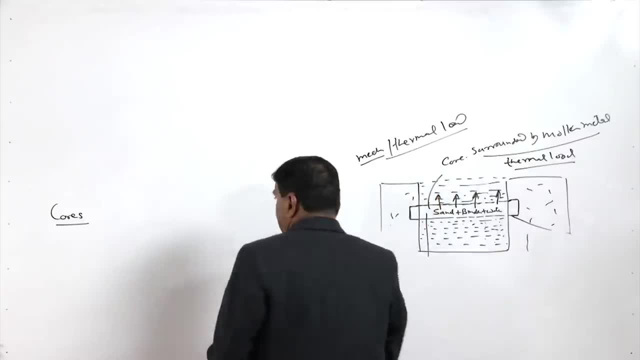 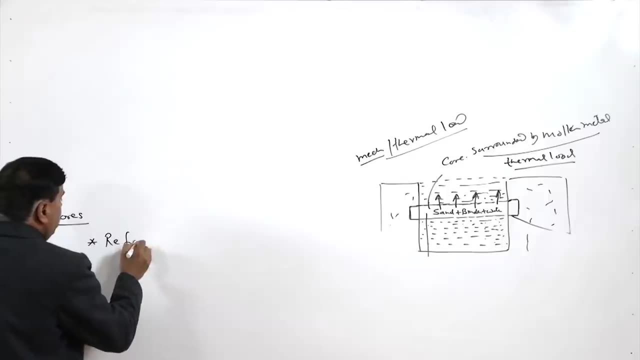 it can perform the function which is intended And what these properties are like. It should be of the very good refractory properties. So refractoriness required in the core is much higher than what is needed for the moulding sand. So higher refractoriness is needed because it experiences much more thermal loading, since 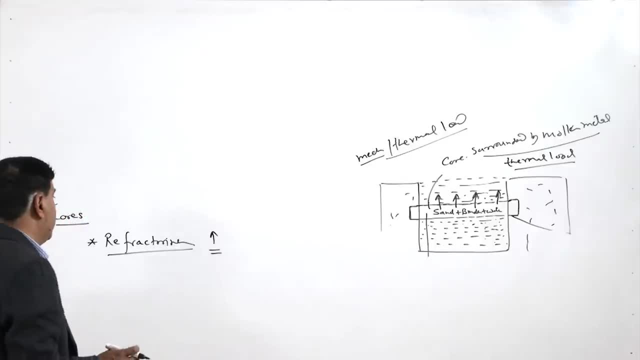 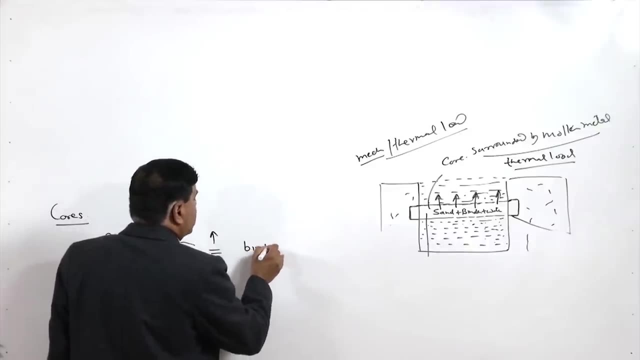 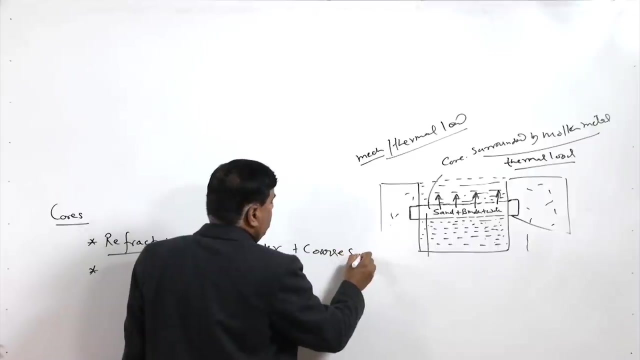 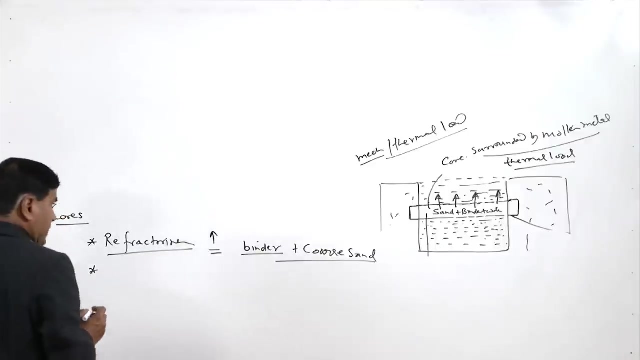 it is surrounded by the molten metal. So normally for this purpose, So normally for this purpose, Mechanic binders- not just the clay- is used and the coarse sand grains are used so that the better refractoriness of the core can be realized. 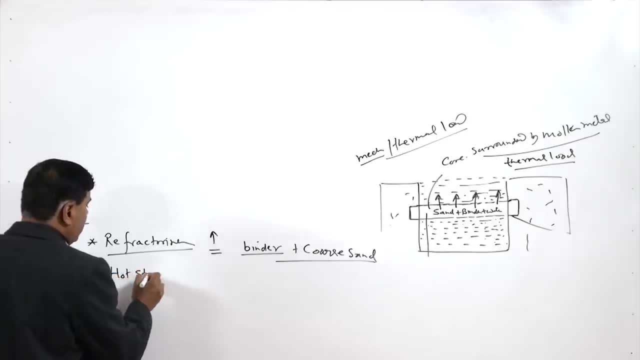 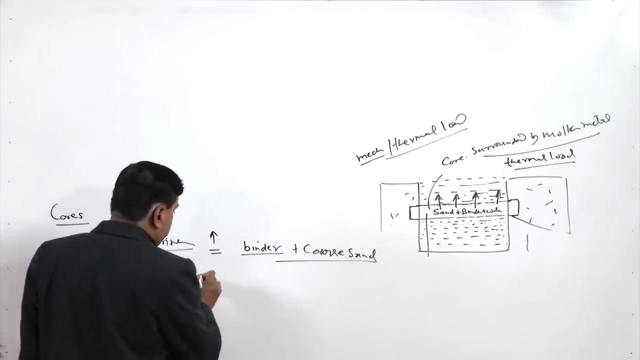 Another is hot strength. hot strength since the buoyancy force acting on to the core, the kind of the mechanical loading which is experienced by the core Are much more severe as compared to those which are experienced by the mould walls, and that is why, at high temperature, hot strength of the core material must be better than what 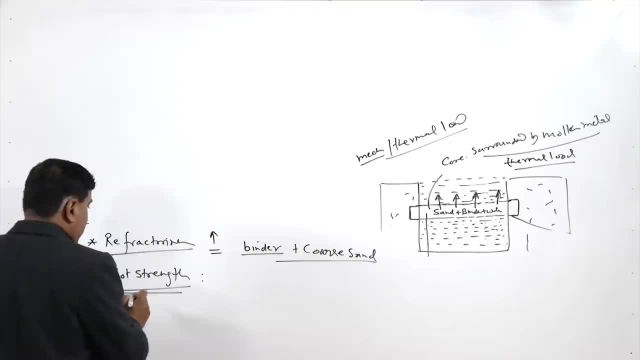 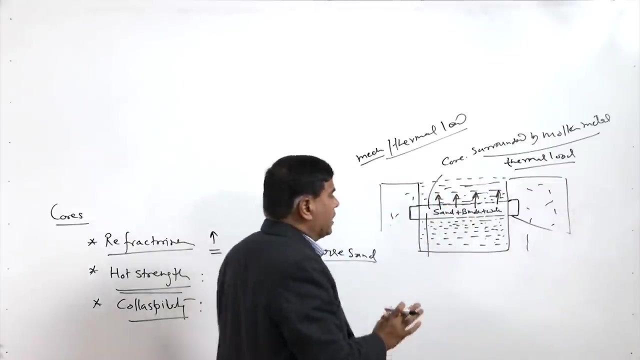 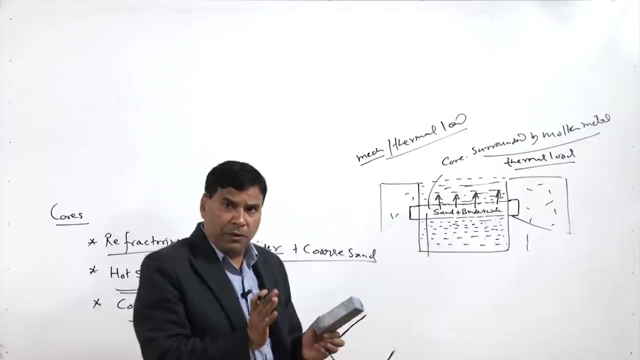 is there with the moulding sand. Then collapsibility, Collapsibility, Collapsibility. So the final material is required because after the solidification, this core will be experiencing the contraction, means the molten metal experiences the contraction and which, and because of that contraction, the core is pressurized from all the sides. 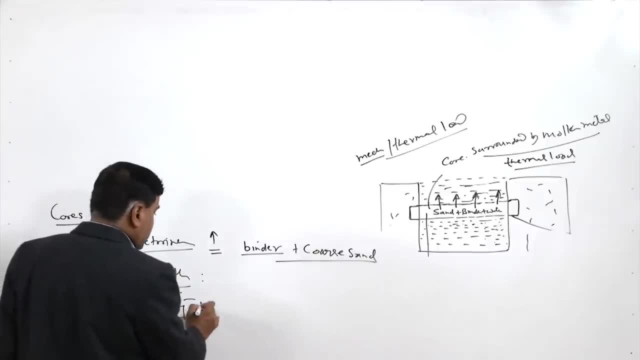 So it is expected that it will collapse under those conditions, and if it does not collapse, then it causes the hot tearing or even sometimes celebrate. So it is expected that. So for this reason. So the material is not workable. 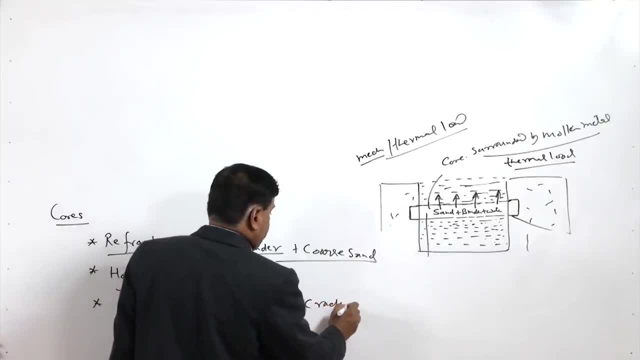 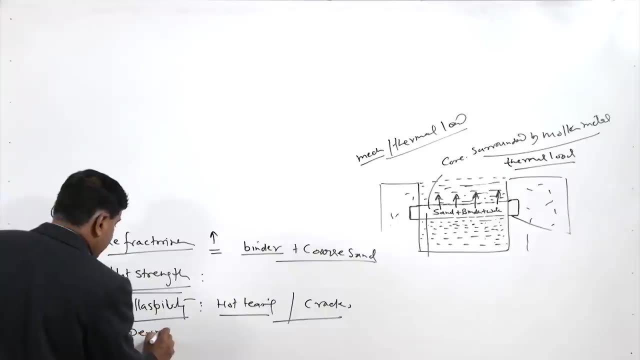 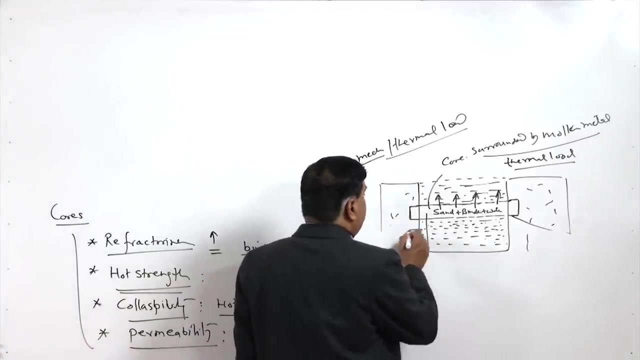 Sometimes the cracks are generated. if it does not collapse, Then permeability is another important property required in the core sand material which is used for making the core, Since in the case of the moulds, there is a lot of area and space through which the gases. 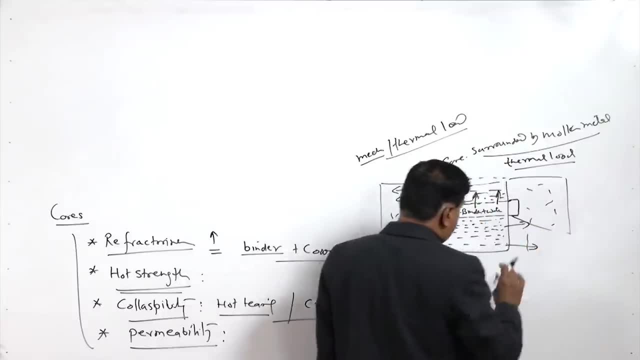 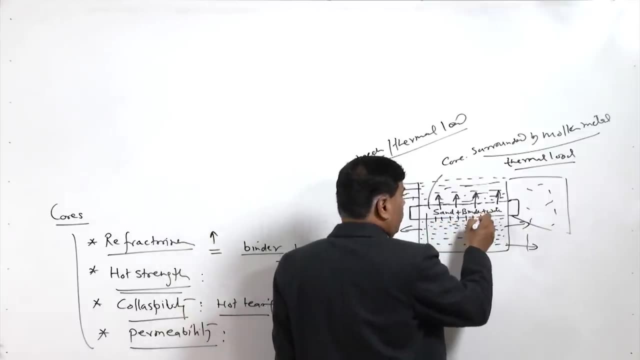 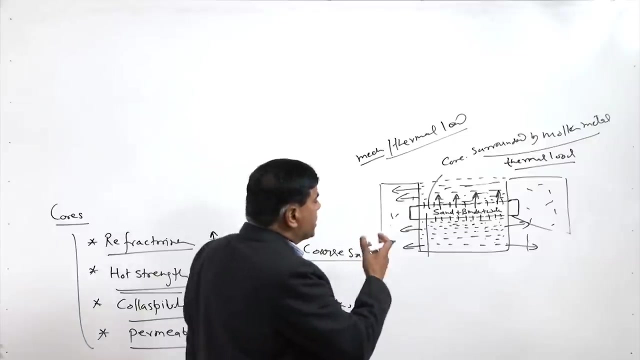 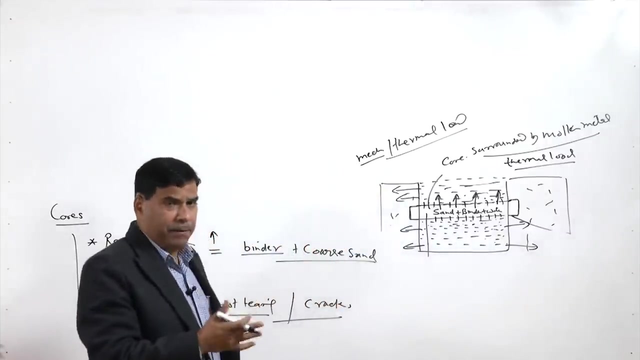 can escape. but in case of the cores, the gases which are produced by the core, molten metal interaction and the removal of the moisture from the core. So these things, these gases, should get passes, enough passes for escaping, so that the porosity is not produced due to the presence of these gases. 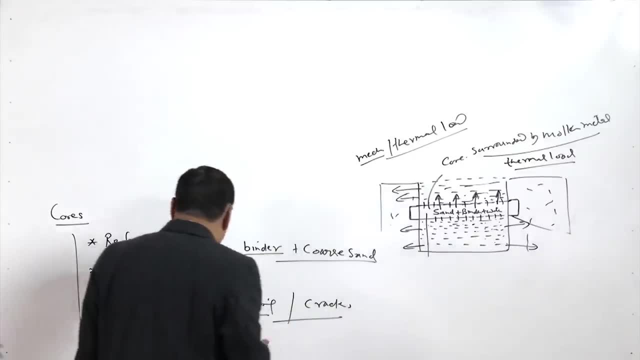 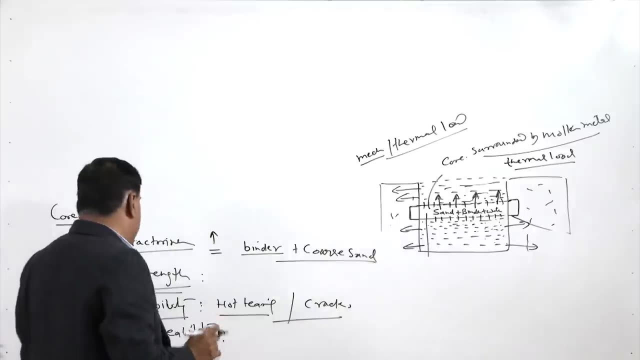 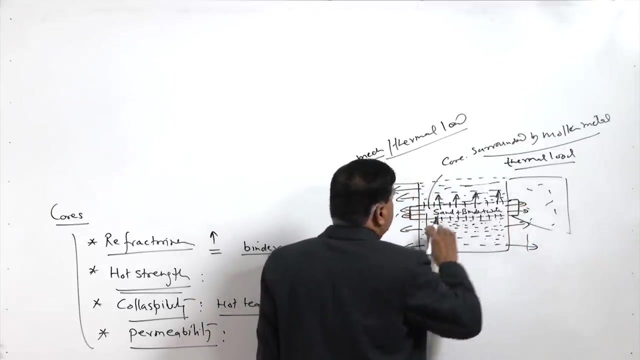 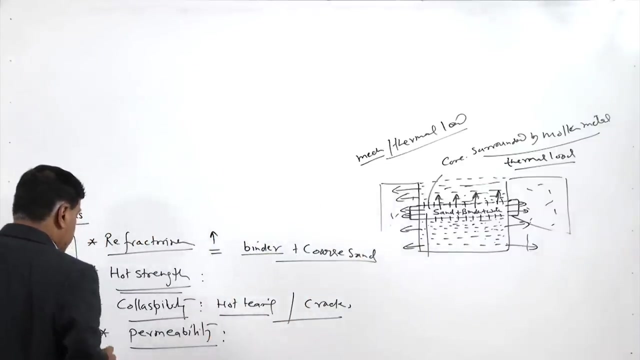 And therefore the permeability of the core sand must be better than what is there with the moulding sand. And here there very limited passage is there for escaping of the gases because from all around the core is surrounded by the molten metal, So good permeability is needed. 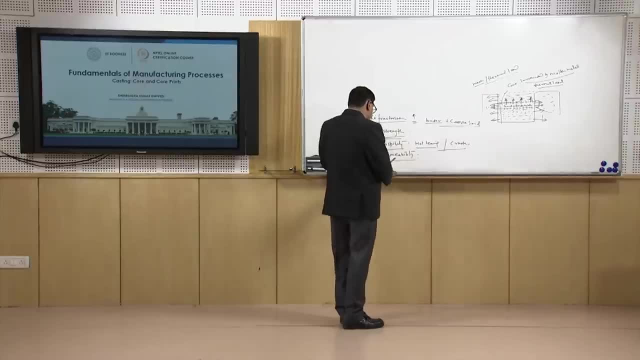 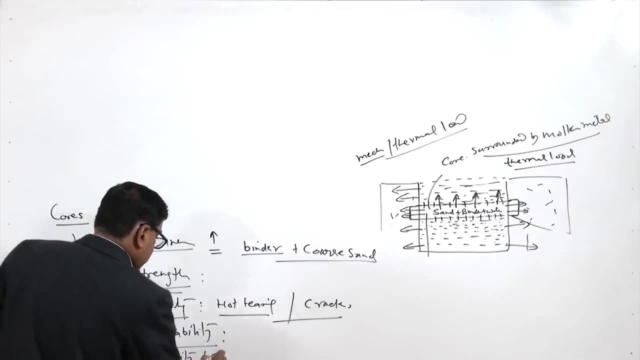 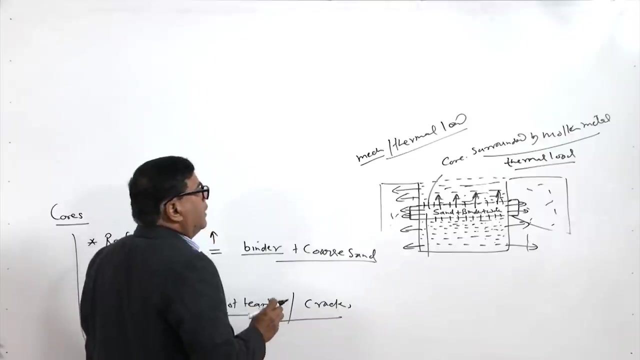 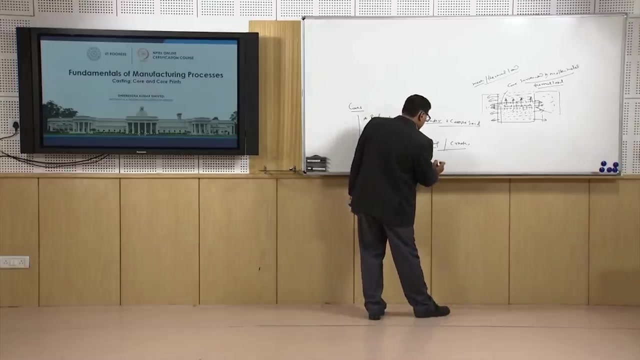 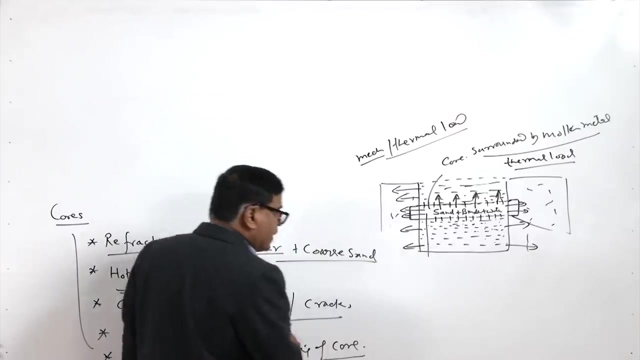 Then another important property which is required is It is a friability and crumbling. friability and crumbling so it should break and it should crumble whenever it is required to remove the core from the solidified casting. So these two properties will be helping the breaking of cores and if it is broken easily. 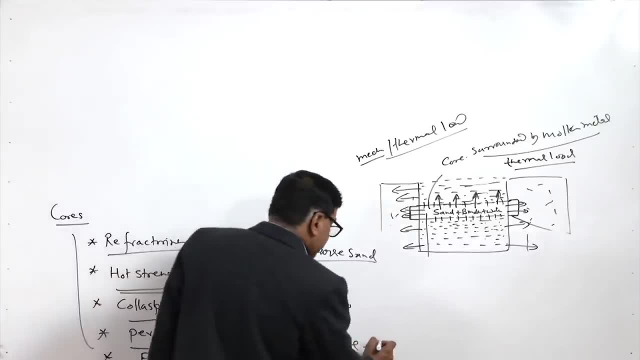 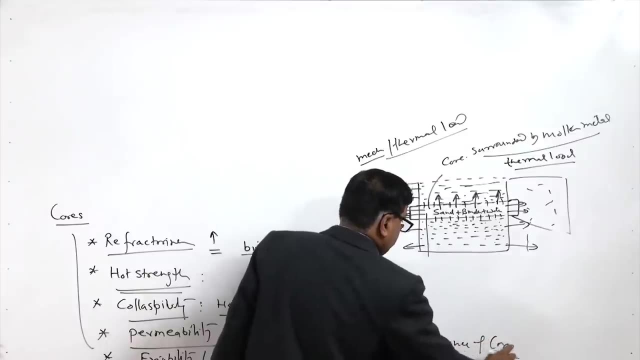 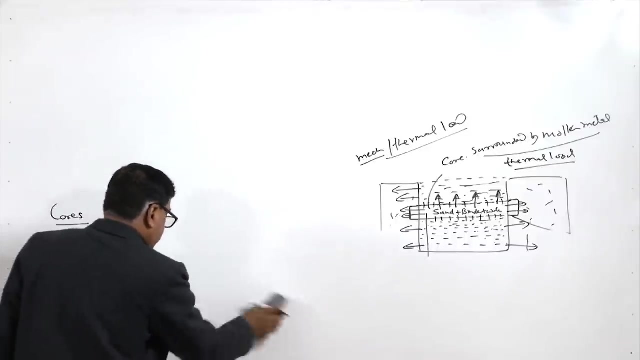 for removal of the core, then the easy clearance of the core will be possible. So removal of the core becomes easier when the friability and the crumbling properties of the core sand is good. So these are the characteristics which are desired in the core sand which is used for. 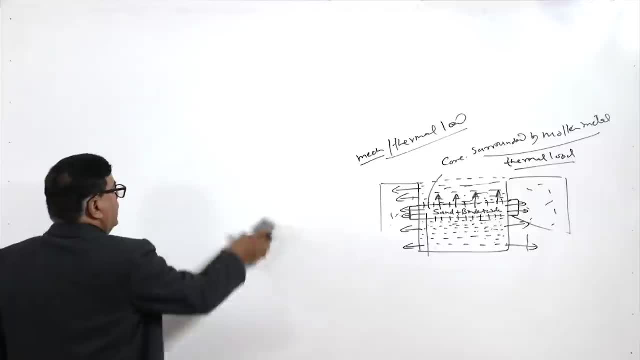 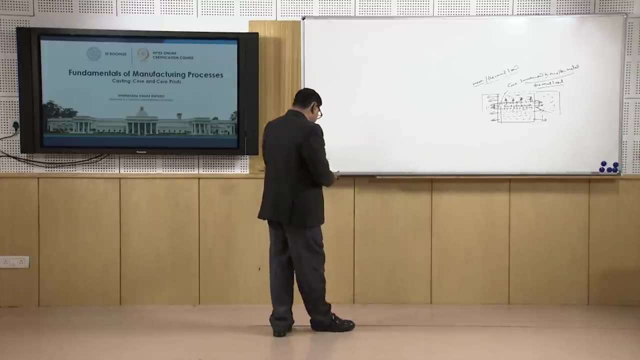 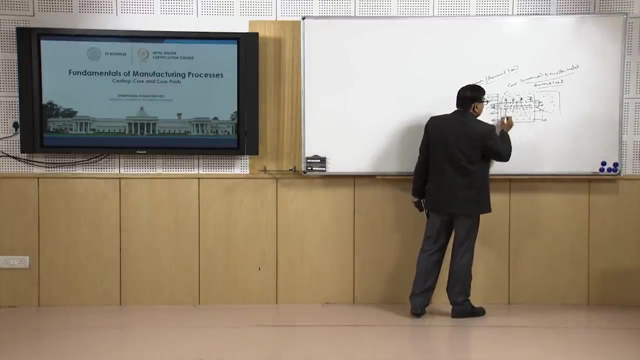 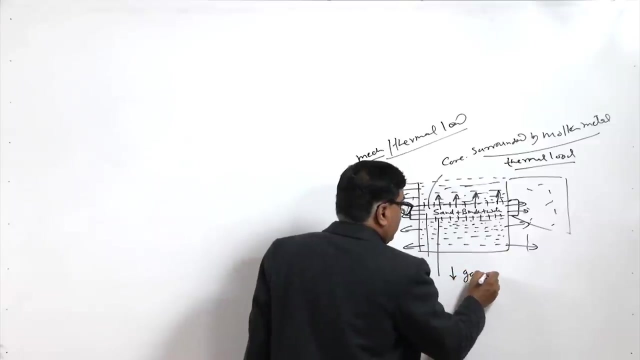 making the moulding Core, not just for the sand moulding but also for the permanent moulds. So another important property is that the low emission, the gases which are generated by the molten metal core interaction, so the less gas evolution tendency due to the core. 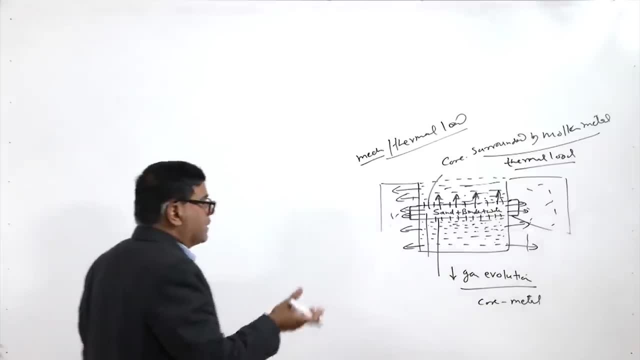 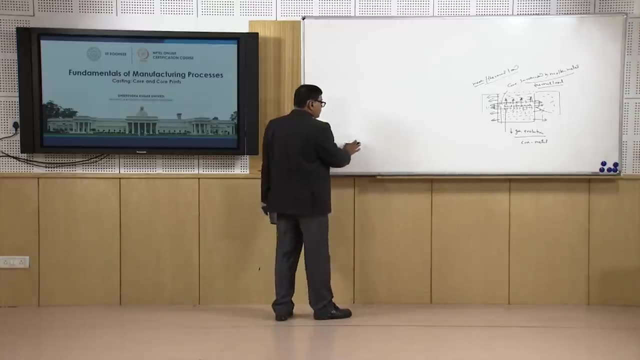 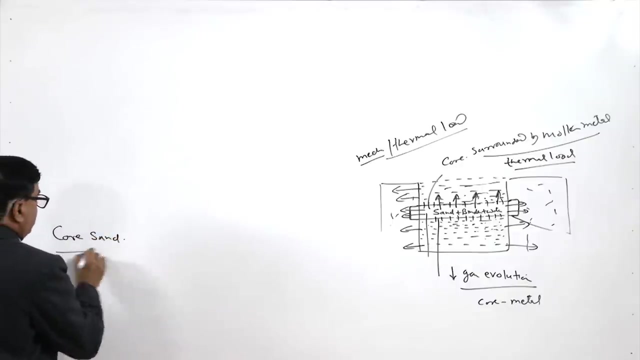 metal. So the interaction at high temperature means the core molten metal interaction should generate as less gases as possible in order to avoid the gaseous defects in the casting. Now we will come to the role of the different constituents. As I have said, core sand is basically comprises silica sand, which is largely free from the 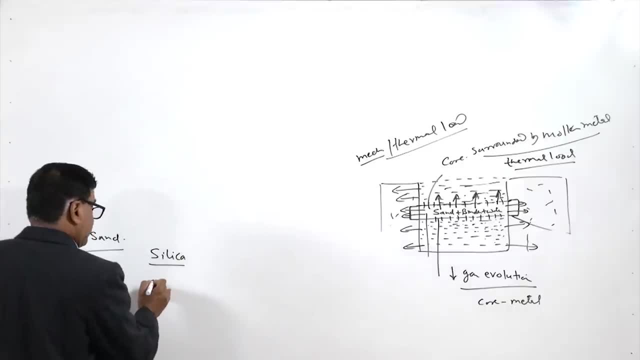 clay and another is the binder and then water. So these are mixed in the different proportions, for example about 1% the binder and 2 to 6% of the water, and the balance is silica, and maybe some additives are also added to achieve the specific set of the properties. 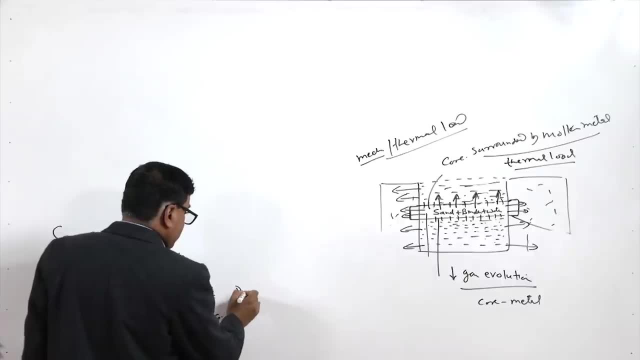 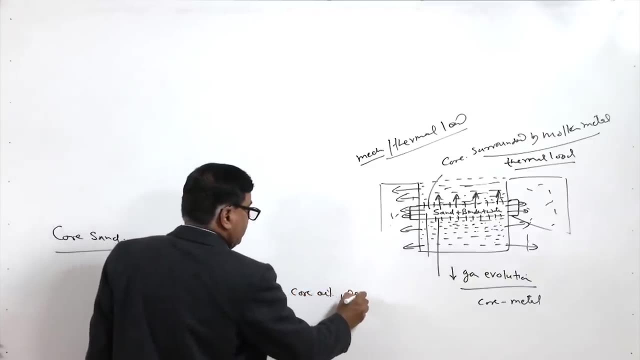 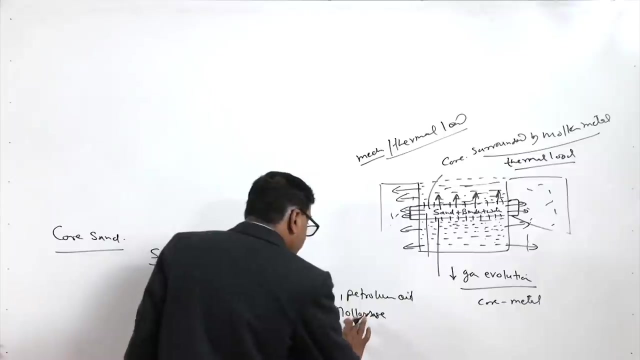 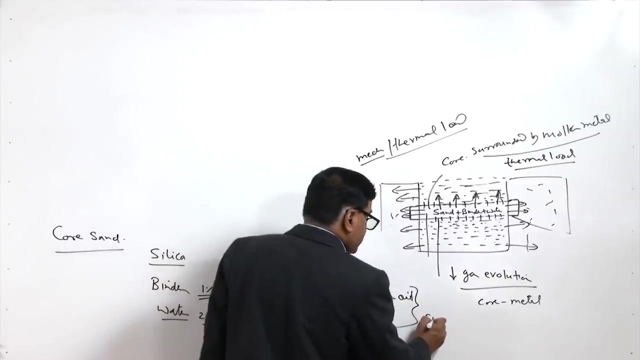 Binders which are used normally. they are like dextrin, core oil, petroleum oil, molysis and linseed oil, Linseed oil and molysis. Okay, So these are the binders which will be able to sustain high temperature as well as they. 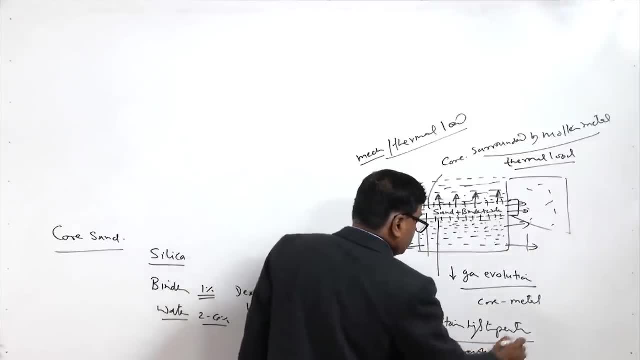 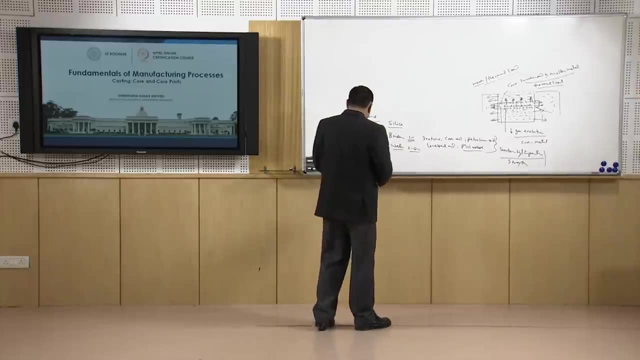 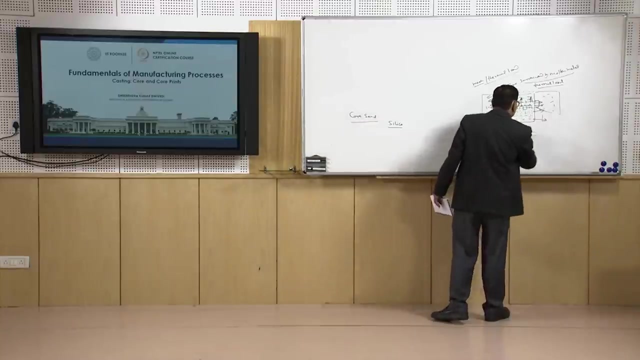 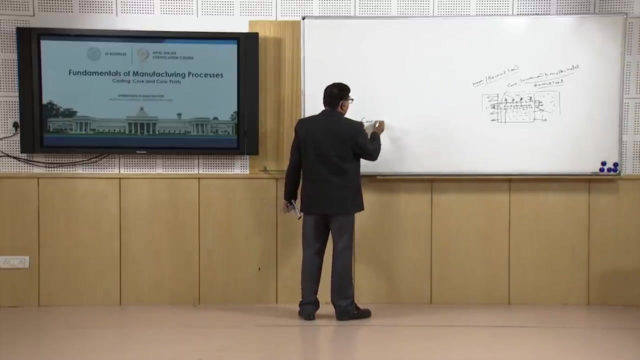 will provide the desired strength to the core so that it can effectively sustain the buoyancy force which will be acting on to the core. Okay, So if we will see the which type of the core, based on the core material or the condition of the core, there are two types. 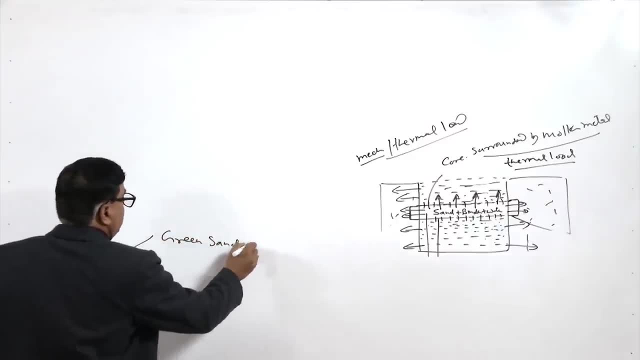 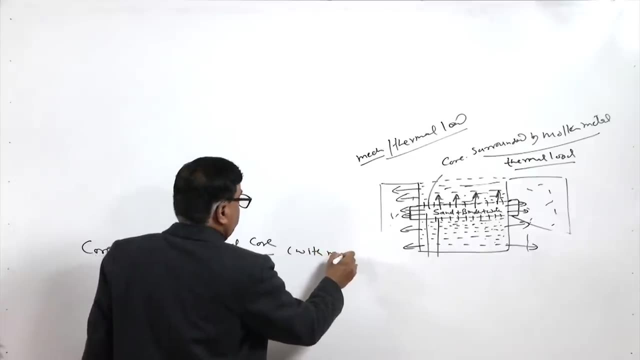 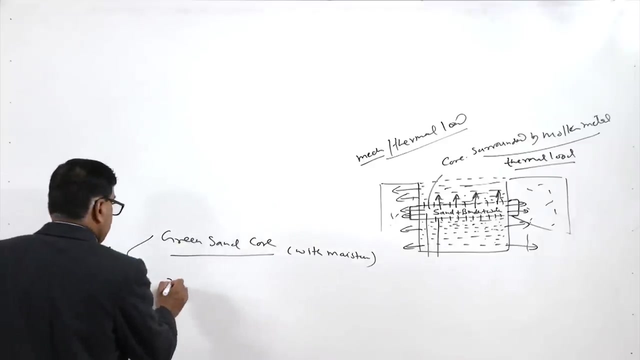 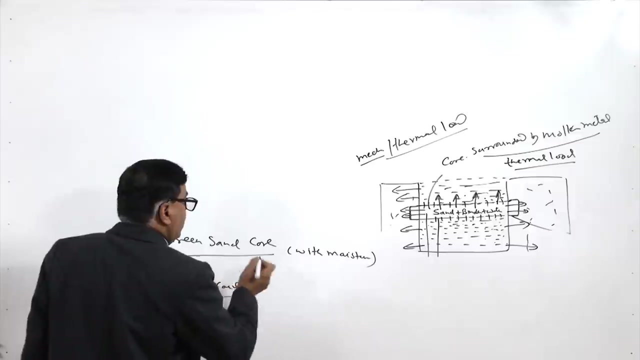 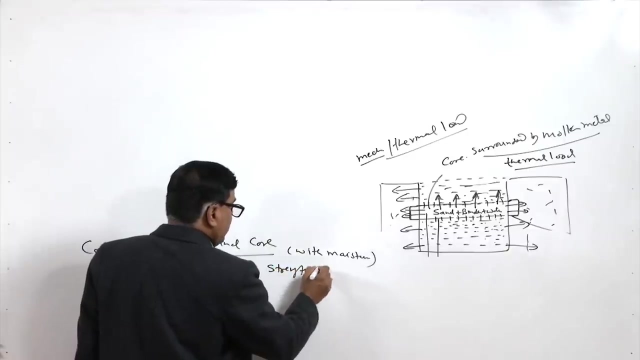 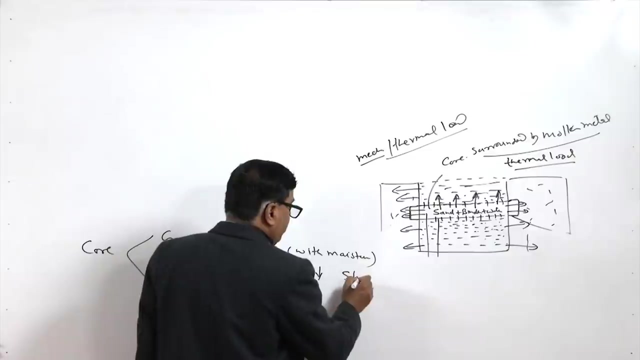 One is green sand core, So this is basically with moisture, Okay, Okay, Okay. So another is dry sand core. So here, since it is with the moisture, so strength of the green sand core is less and therefore it cannot be used, means it is normally used for producing the shallow features. 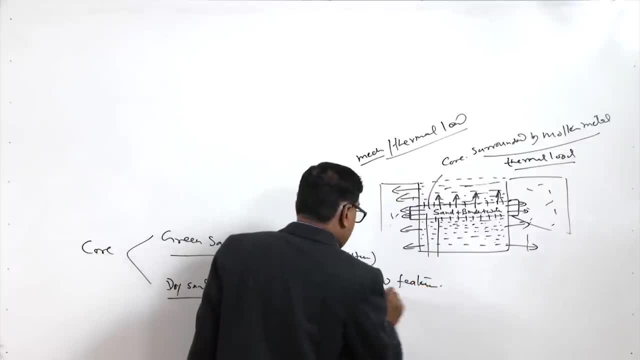 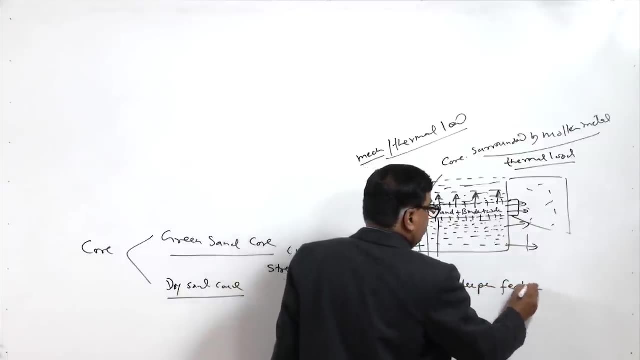 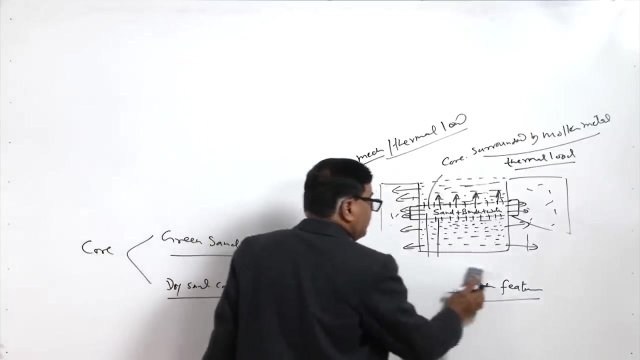 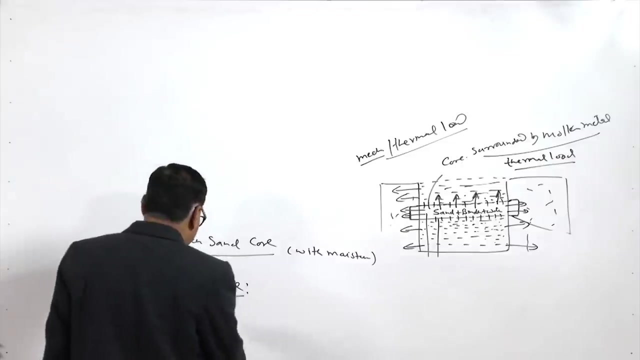 Shallow features. Shallow features Because when the efforts are made for the deeper features, you see, the cores will have tendency to get break. Therefore, for the limited depth features are produced with the help of the green sand cores. So, in order to strengthen, the green sand cores are baked or heated at one side. the 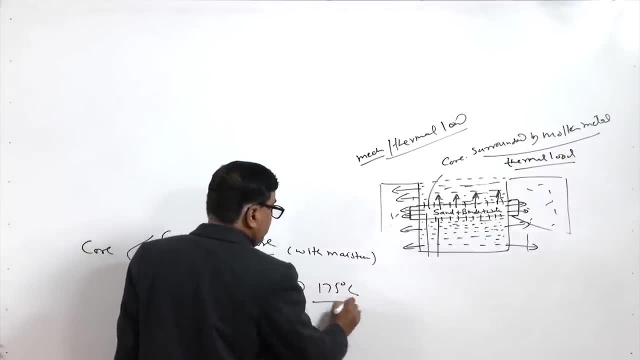 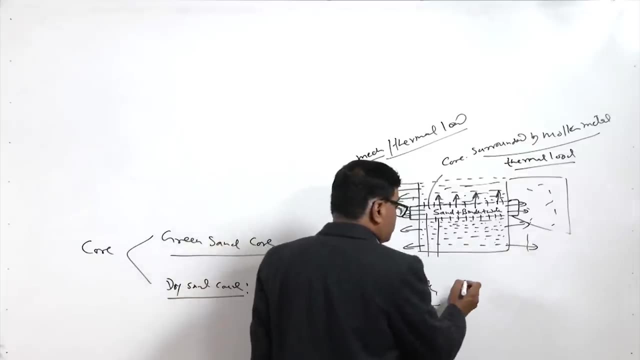 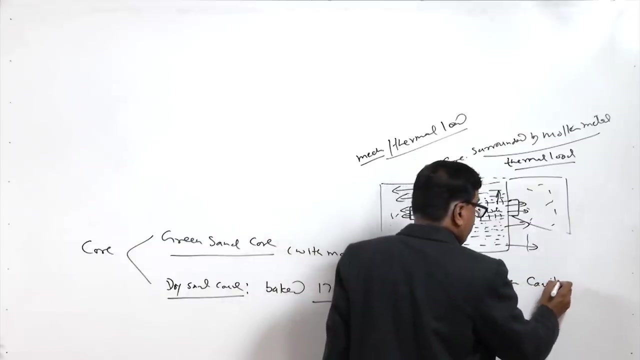 green sand cores are heated at 175 degree, So this helps to increase the strength, and that is how it can be used for making the deeper cavities as well as the thinner sections of the finer sections. Otherwise, the green sand core will not be used. 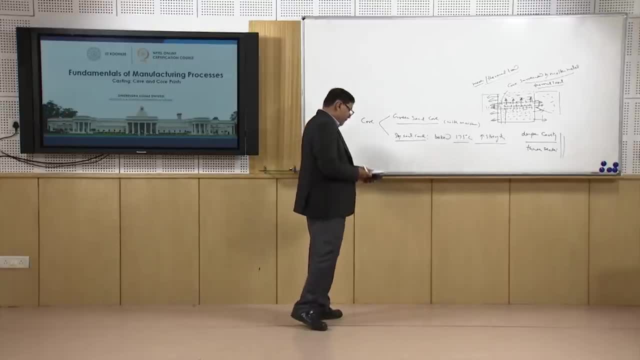 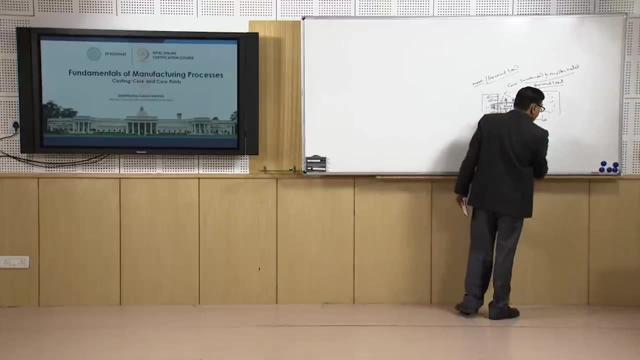 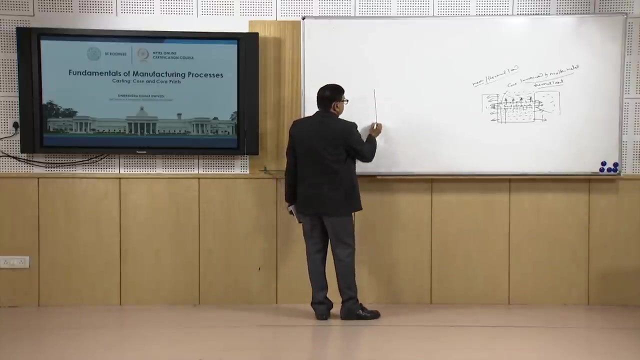 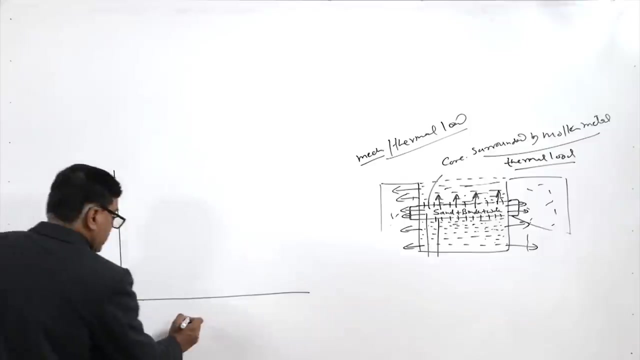 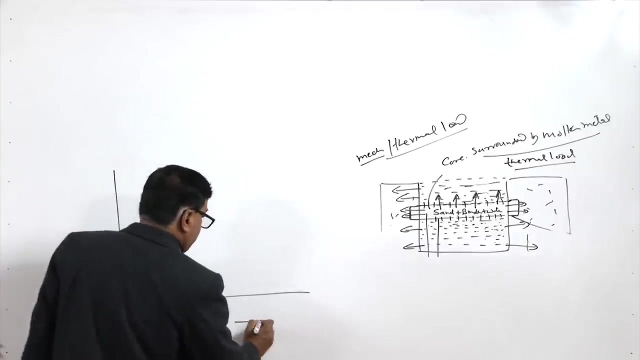 Okay, Okay, So this will be breaking down. if it is used for the thinner sections and for the deeper or high aspect ratio, the cavities, Then there is a typical diagram which shows that how there will be change in the properties of the core with the change in the ratio of sand and the oil which is used as a binder. 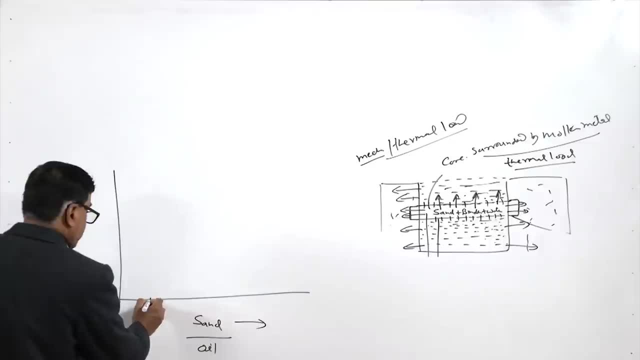 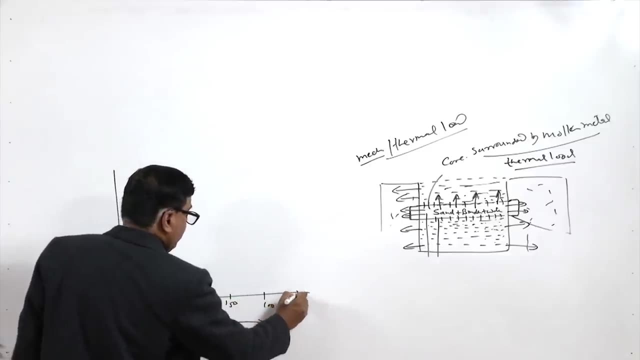 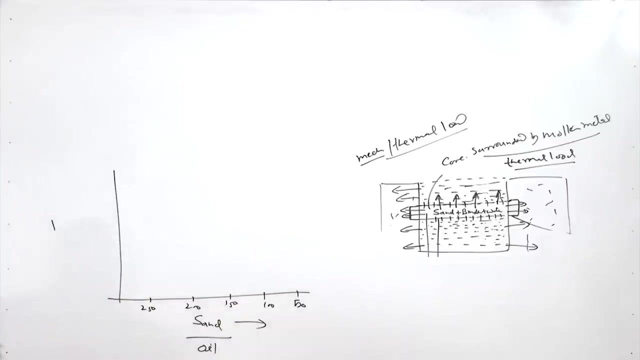 in the for making the core. So like, say, the ratio is 250,, 200,, 150,, 100 and 50. What it is showing that the amount of the sand is decreasing and the fraction of the core is increasing, and on the y-axis we have the properties like permeability, strength. 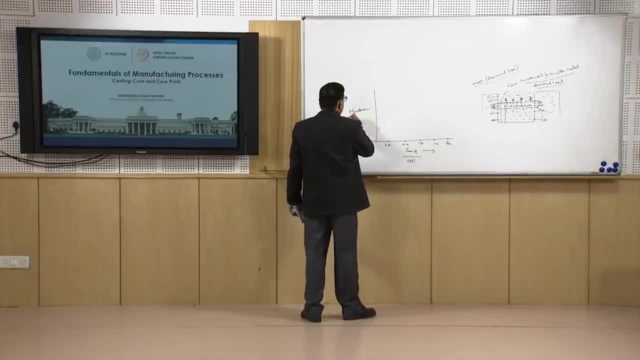 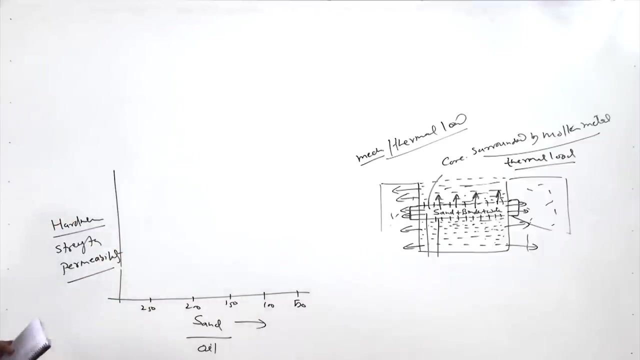 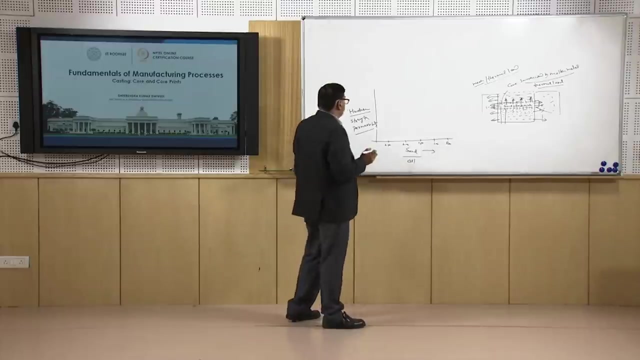 and the hardness. So how these three will be changing: permeable hardness, strength and permeability. So, as we can see, with the increasing content, of the binder basically will be holding the sand grains together firmly and reducing the pores between them. So basically there is a tendency for little decrease in the porosity. 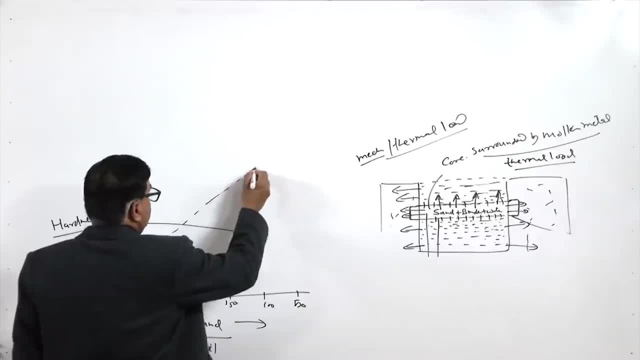 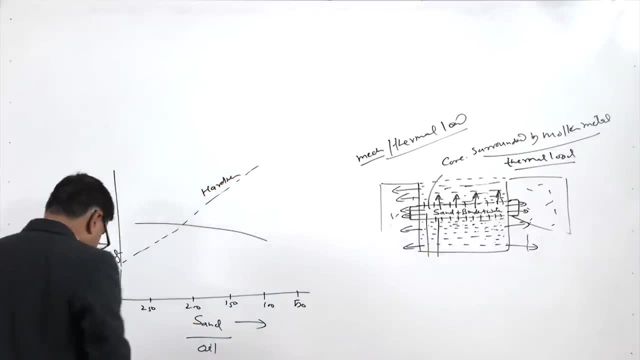 Okay. So the hardness continuously increases with the increasing concentration of the binder and the similar trend is also observed. it is not linear like the hardness, but there is a significant change in the strength with the increase in the fraction of oil, or you can say reducing fraction of the sand. 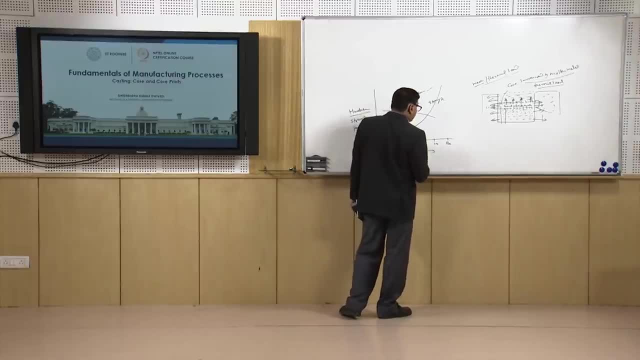 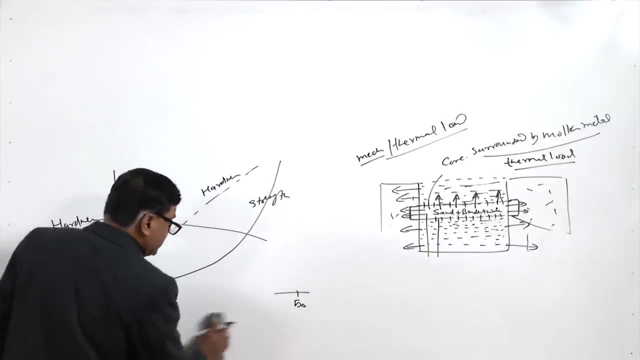 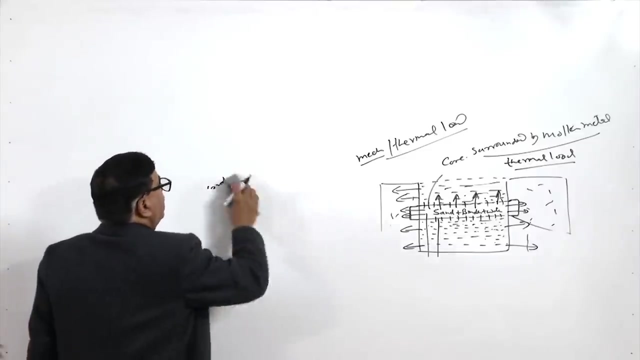 Okay, So there is a significant change in the strength of the sand to the oil, or the binder ratio. So, as per the requirement of the strength, permeability and the hardness, the suitable ratio of the core of the sand and the oil can be used in order to have the properties. 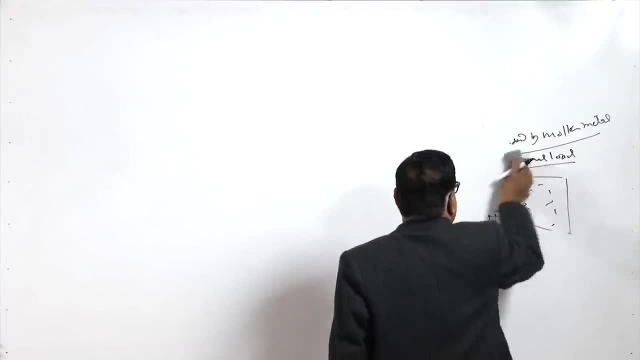 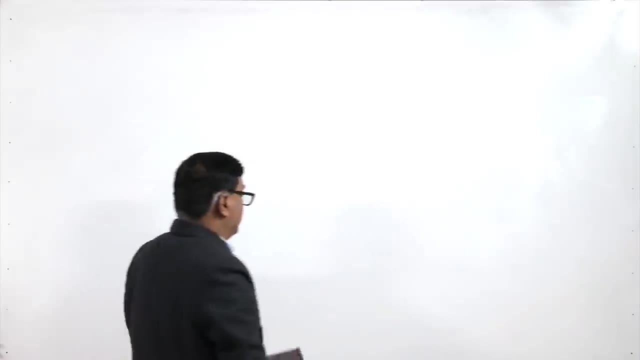 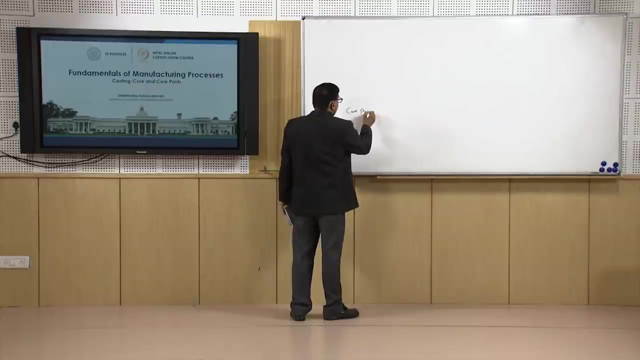 which are desired in the core for the desired purpose of strength and the hardness. Okay, So this is the point. So this is the point, So this is the point In the hardness. Now we will be talking about the core print. 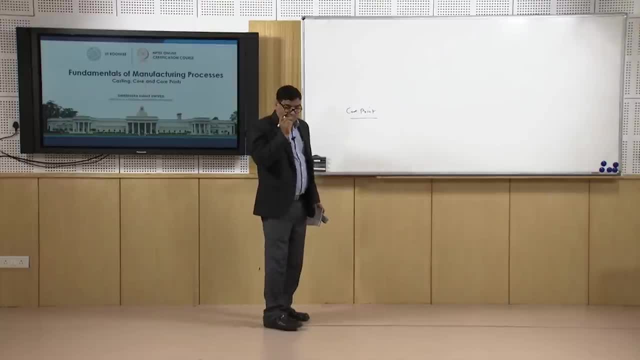 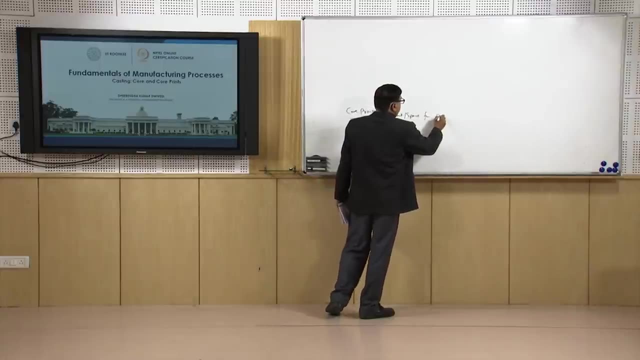 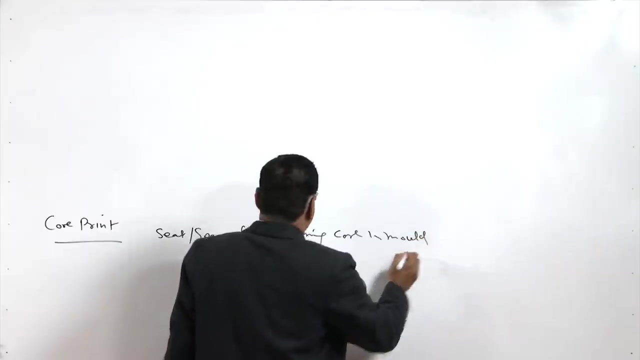 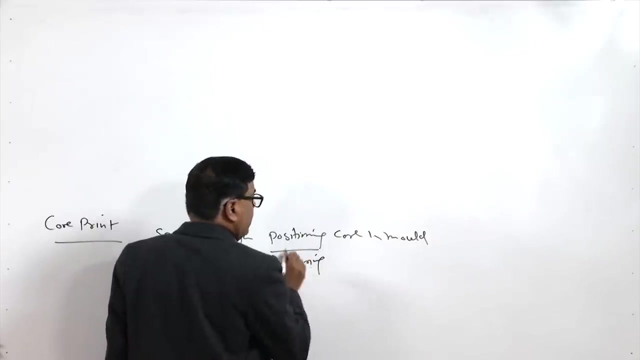 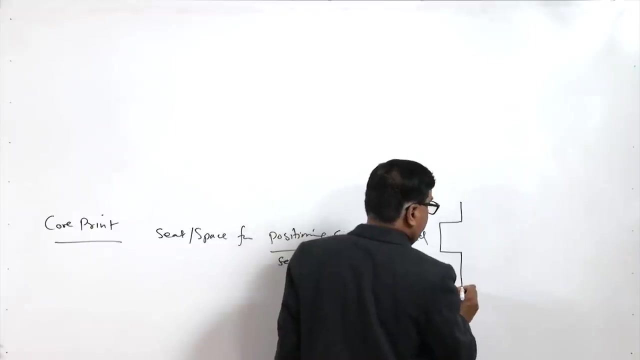 Core print. basically it provides the seat or the space seat or space for positioning the core in the mould. So positioning as well as securing, So they are also present there. So the core is the space for the mould. securing it is to be held properly, securing into the moulds say so this is the core print. 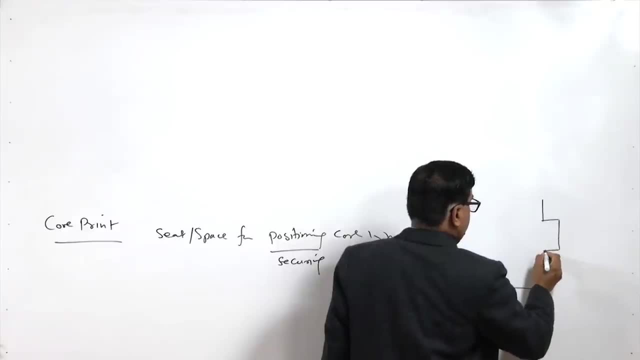 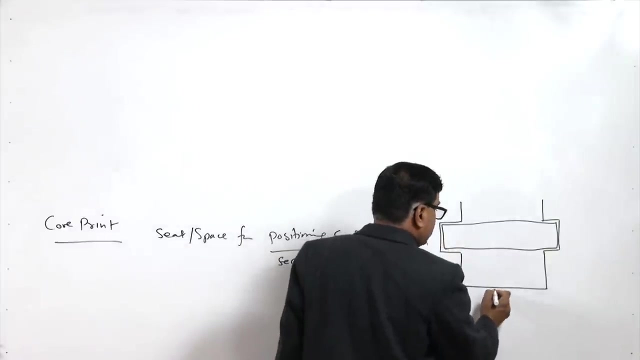 this is the cavity, this is the core print. So here, this is the location where the core will be placed. okay, So, when it is placed properly, this is one configuration. there can be another configuration like this if the core is to be placed vertically. 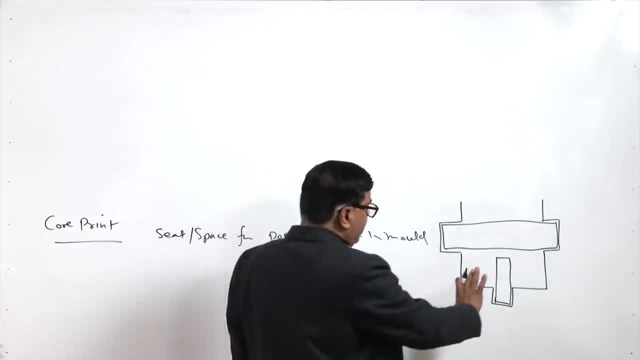 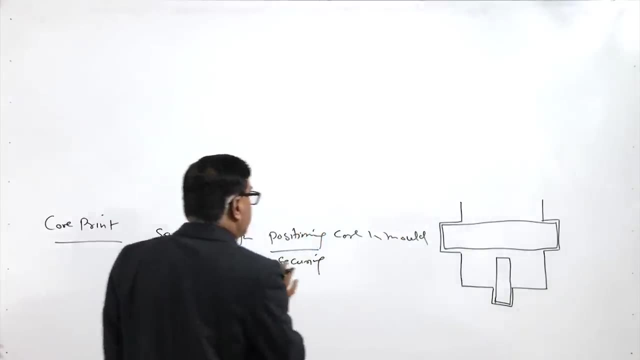 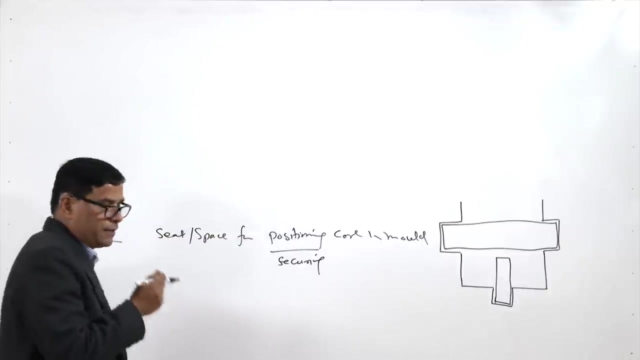 So the purpose is that the core is placed in such a way that it retains its position and its position is maintained and it also carries the metallostatic pressure without disturbing the position of the metallostatic pressure of the molten metal, without disturbing the position of the core. 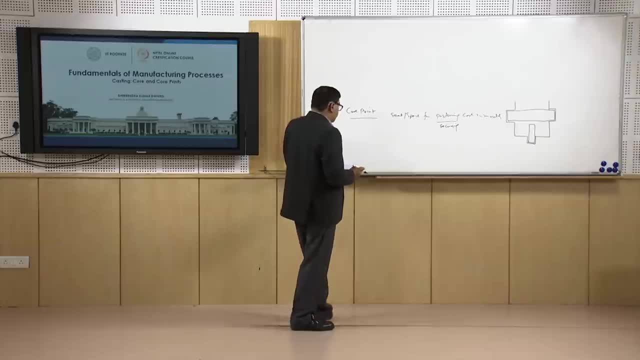 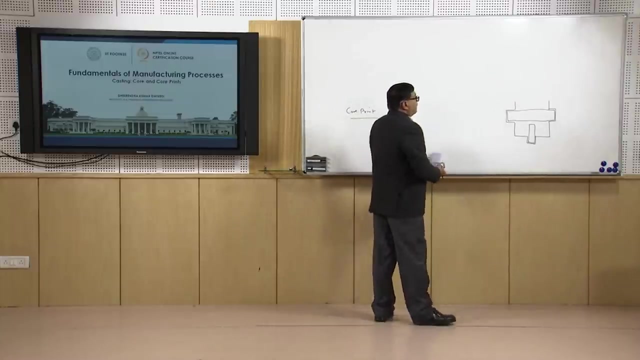 So, for this purpose, what we need, that it not just positions, but also secures the core in its position, and for that it is necessary to consider the forces acting onto the core, so that you can identify what size of the core print is to be used. 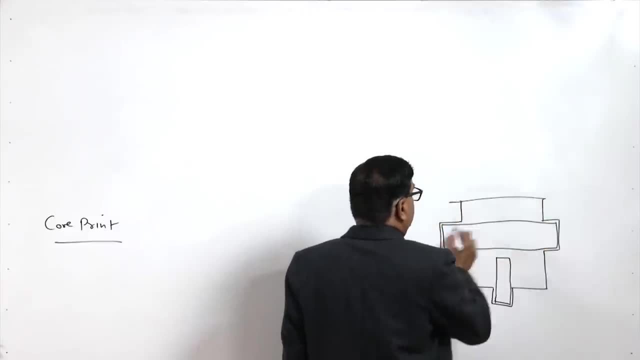 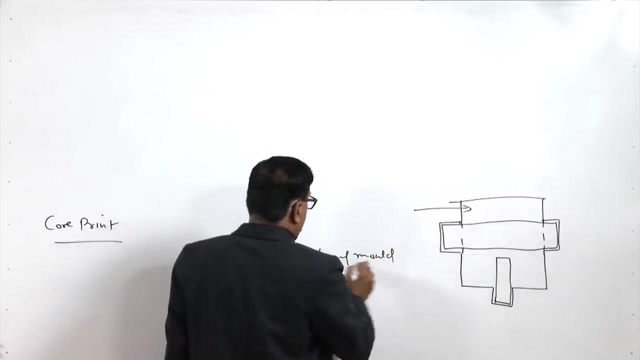 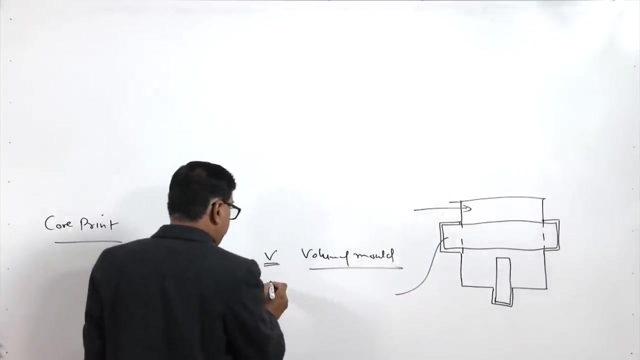 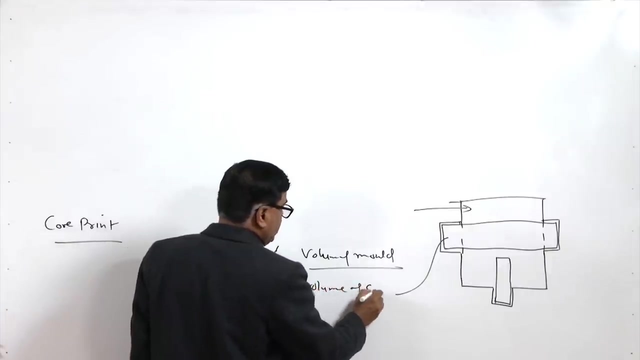 So considering this example, like, say, the volume of the mould, This is the mould, basically, and the volume of the mould is V and the volume of the core, so this is capital V. and then we can say small, v is the volume of the core which is placed. 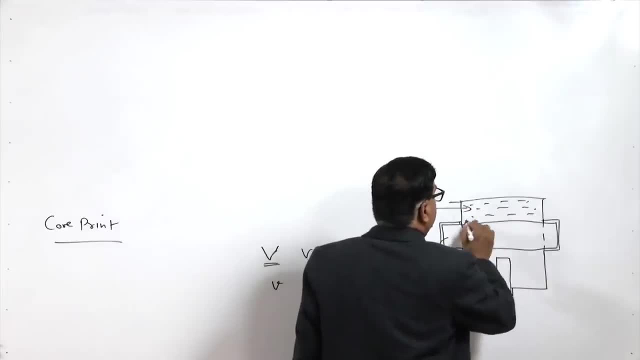 So when the molten metal is filled in the cavity, Since the molten metal is of the higher density. so this is what we can raise, just to simplify, and this is the volume of the core, So small v, and the capital, V for the volume of the mould. 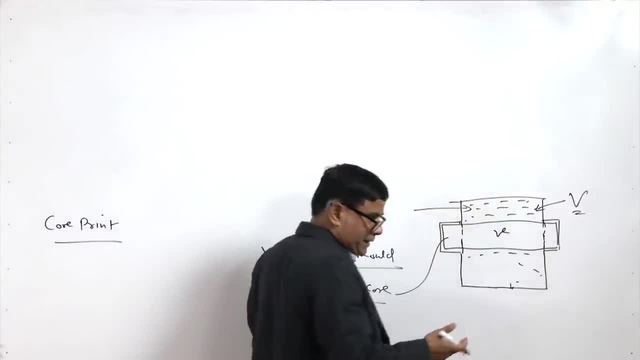 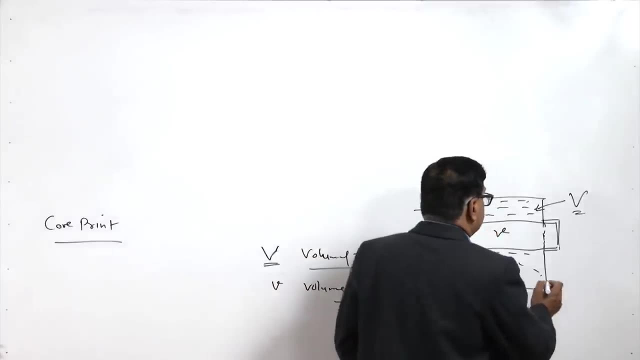 So the buoyancy force due to if the molten metal density is higher than the density of the core. So the buoyancy force due to if the molten metal density is higher than the density of the core, So this is low and the density of the core is normally considered like 1.65- 10 to the. 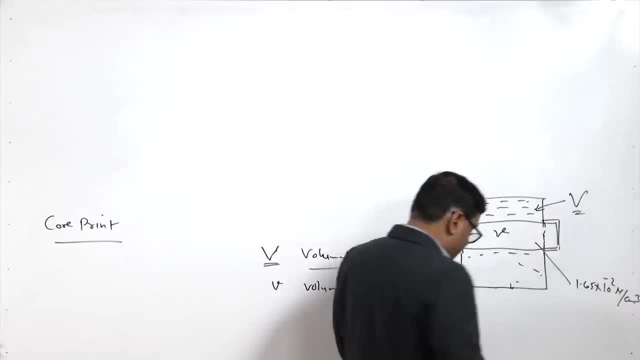 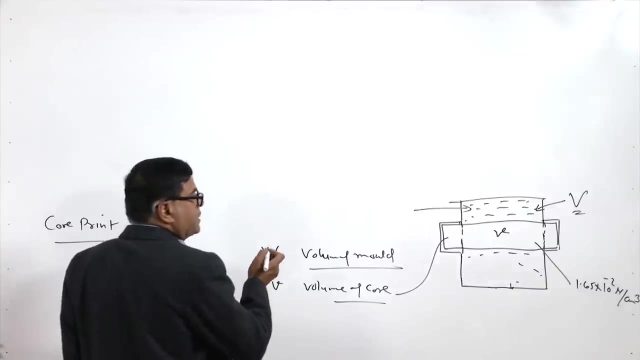 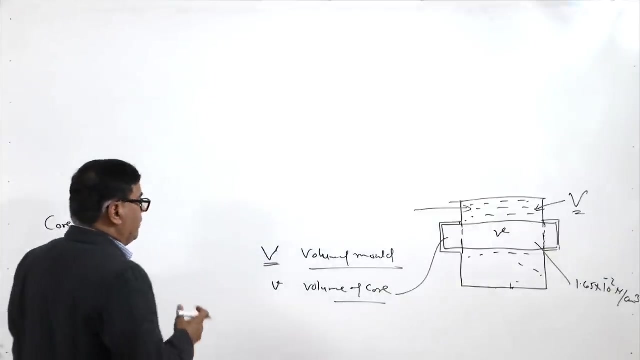 power minus 2 Newton per centimetre cube. So this is the typical value of the density of the core. So if the density of the molten metal is high, metal which is being processed by a casting route, if that is high, So rho is the density. 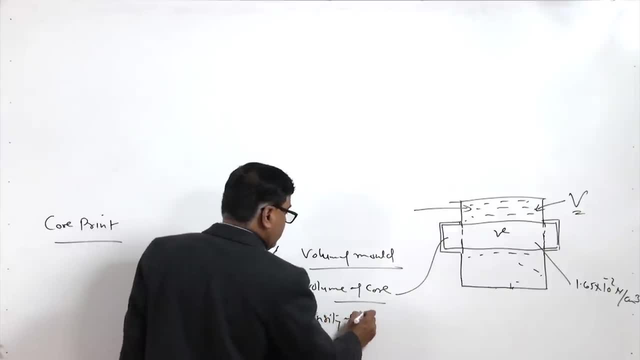 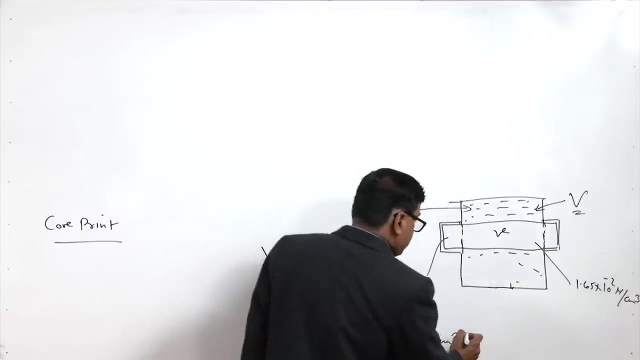 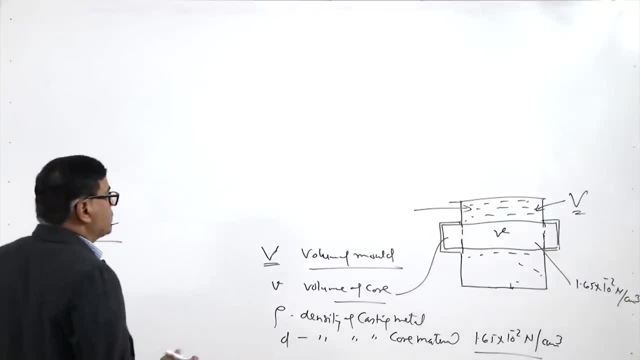 So to determine the forces. So, since the density of the most of the time, So the density of the molten metal, is high, So the buoyancy force which will be acting in upward direction, B U Y, buoyancy force P say will be acting, can be determined from the volume of the volume of the core into 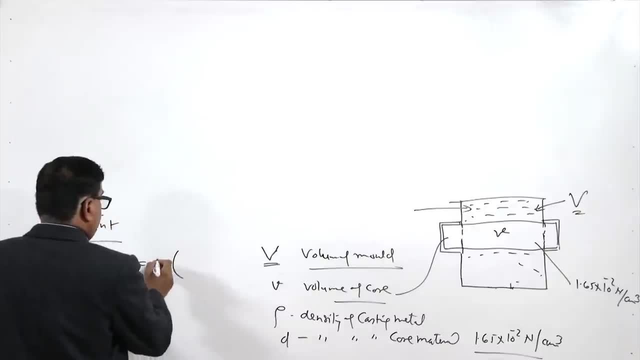 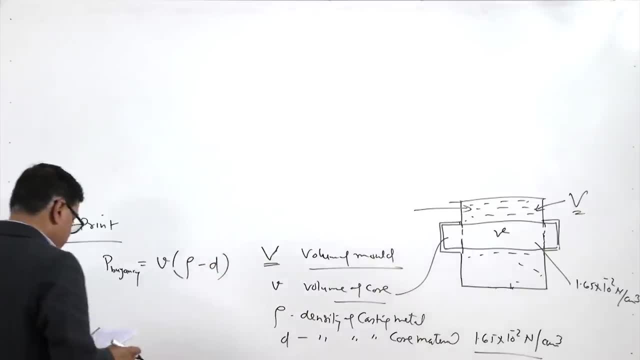 Then the density of the of that we see very clearly for sure now what we are means course, and so this is what is used for determining the buoyancy force which will be acting. So we know the density of the course and material from the calculations for such cylindrical 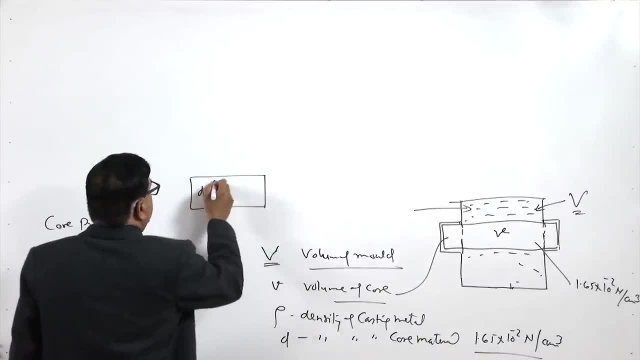 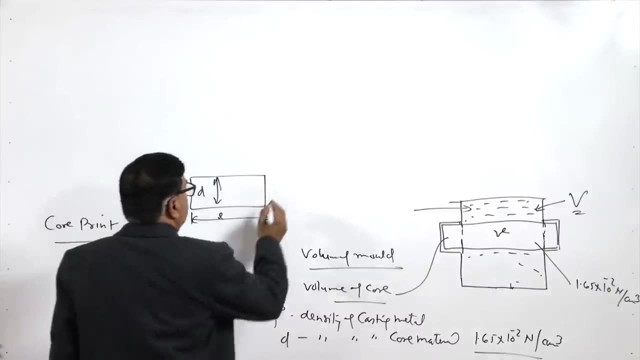 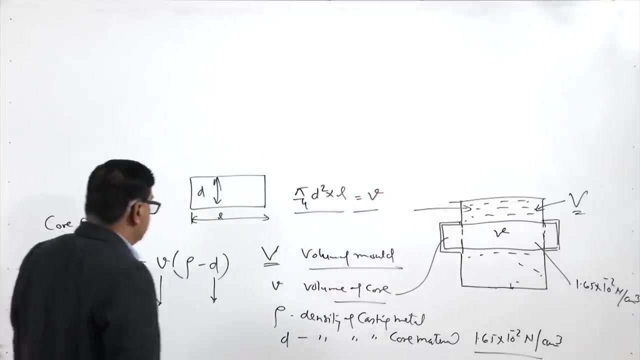 shape of the core if the diameter is D Once and the length is L, which is there in the mould cavity. So pi by 4 D square L can be used for determining the volume of the core. So, once if you know the volume of the cores and the volume of the density of the core, 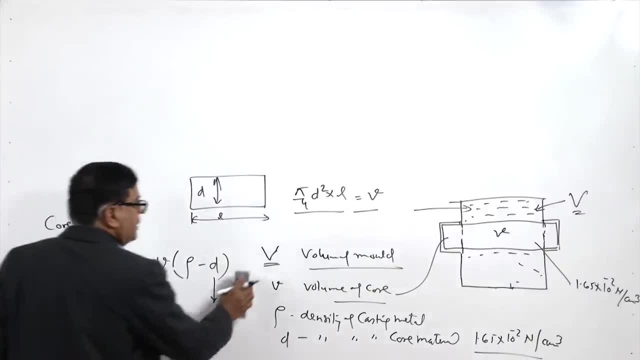 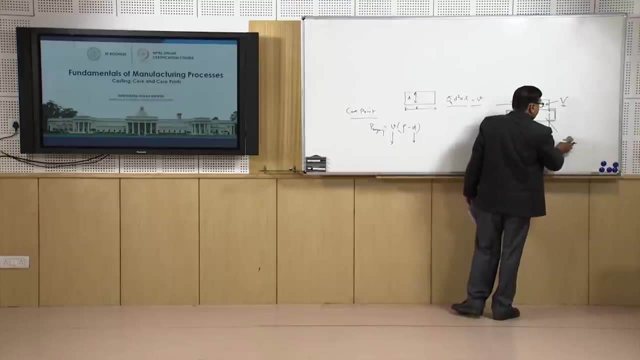 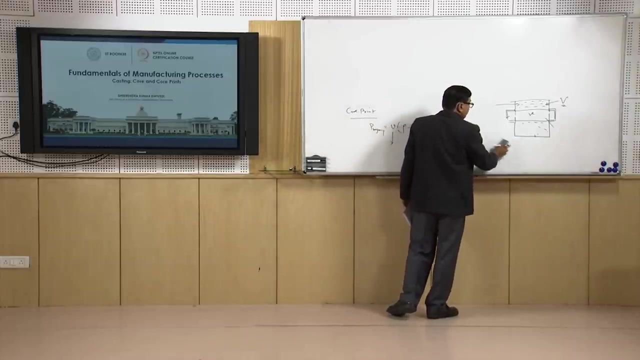 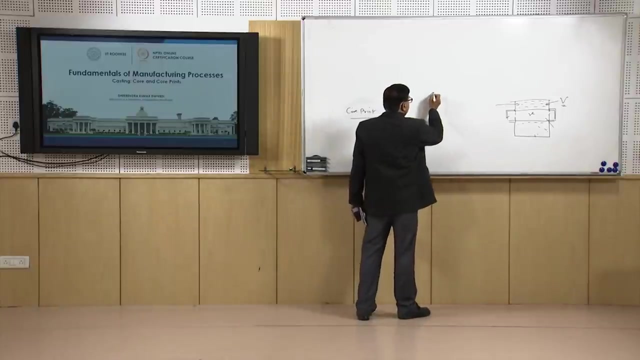 material. to calculate the buoyancy force we just need the density of the casting metal or metal which is being processed by the casting route. So the difference in density will be governing for a given core size and for a given cores and material. the density of the casting metal will be significantly governing the force. 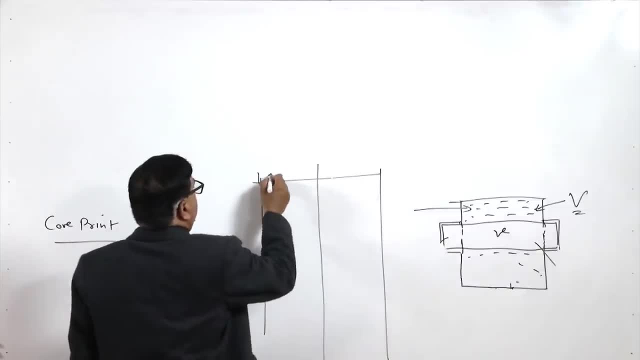 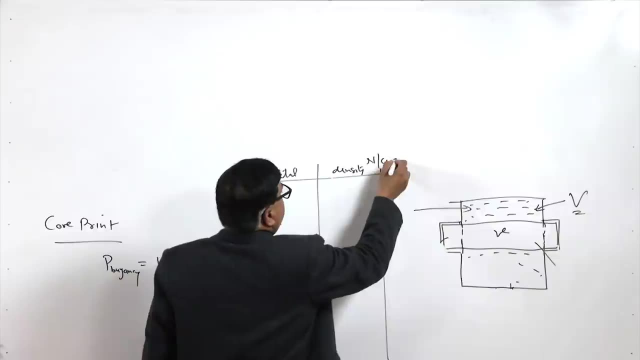 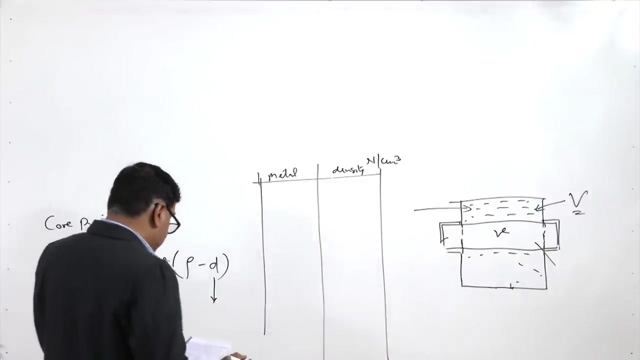 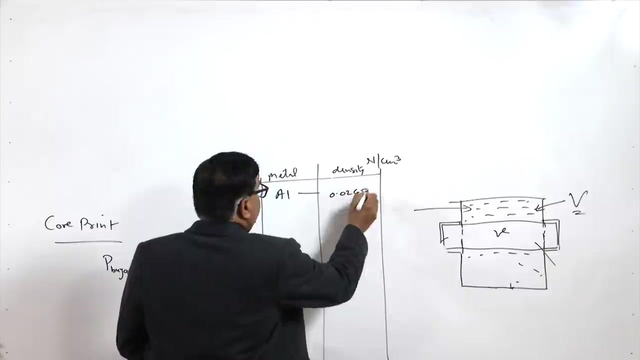 which will be acting. So, considering the metal here and the density here, Newton per centimetre per second. So I will be writing the density of the common metals which are processed. say, for aluminium, it is a 0.0265, for copper, 0.0875. for magnesium, 0.0171. for zinc, 0.071.. 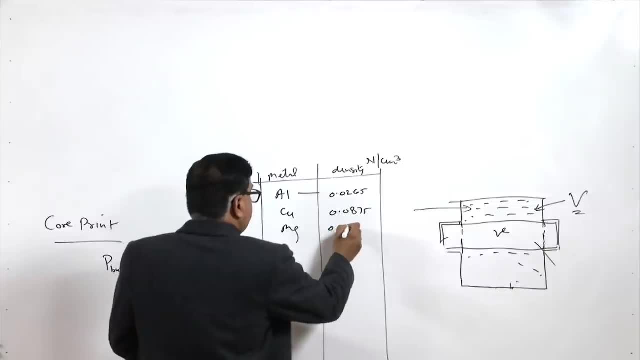 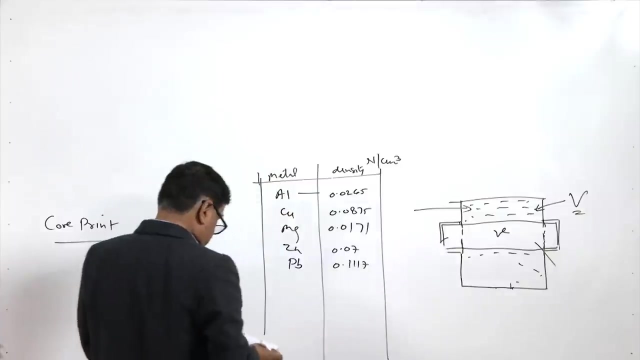 So this is 0.0265 for copper, 0.0875 for magnesium, 0.0171 for zinc: 0.071.. So this is 0.071 for copper, 0.071 for lead: 0.1117. sorry, 3 for steel. it is a 0 point. 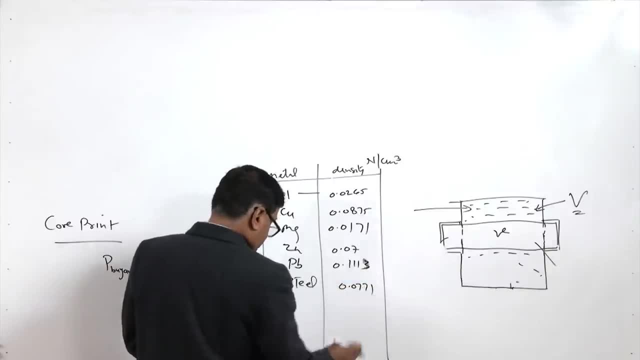 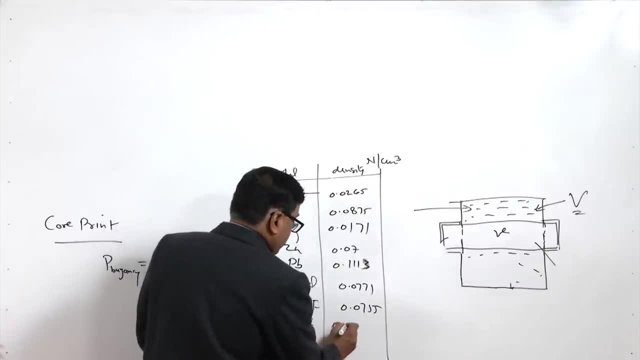 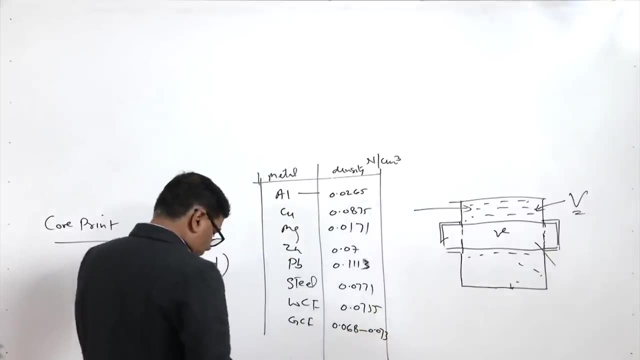 So this is 0.0775 and this is 0.0775.. And this is 0.0775.. It varies over a range like, say, 0.068 to the 0.073, and for the moulding sand, not for the. 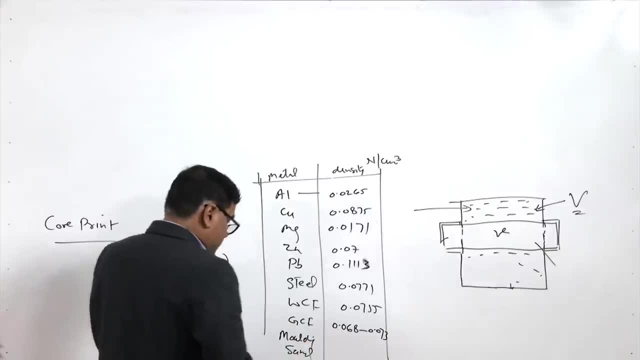 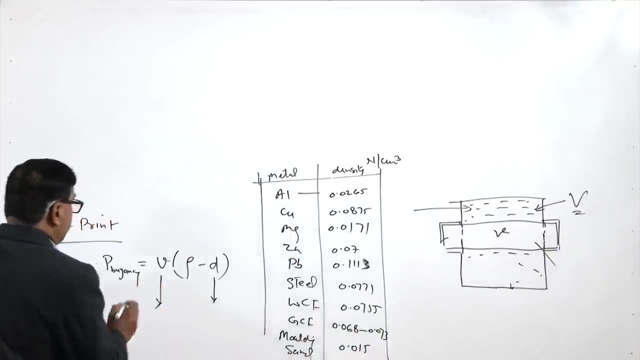 cold sand, but for the moulding sand it is of 0.015.. So this is what can be used for determining the magnitude of the buoyancy force. So buoyancy force B, U, Y, buoyancy force can be determined using this. 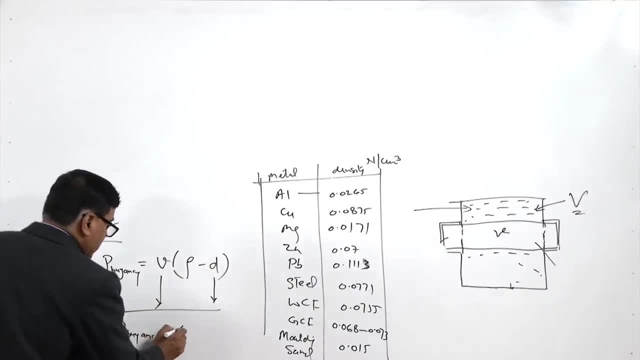 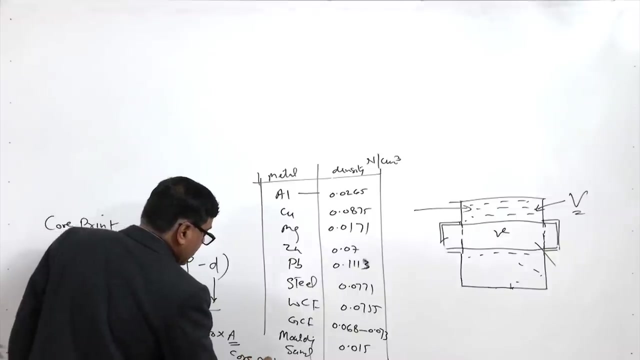 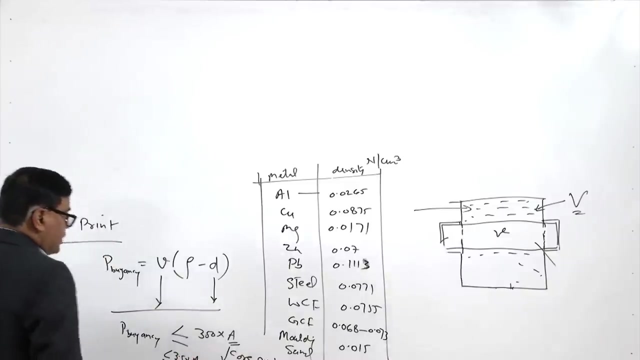 If this buoyancy force comes out to be less than or equal to the 350 into A. A is the core print area, So here it is in mm square. If you want to write that in centimetre square, then 3.5 into A in centimetre square. 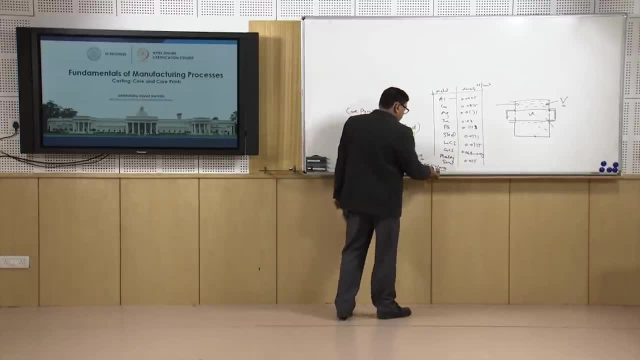 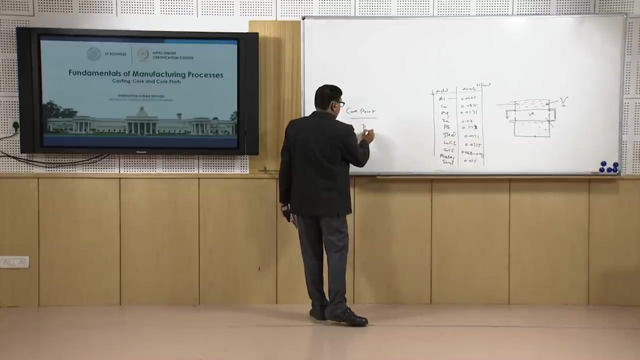 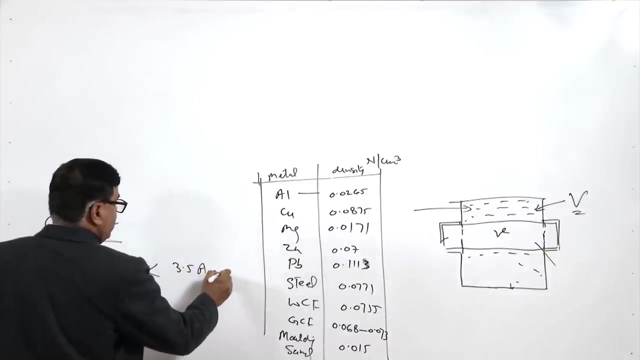 So A basically represents here the core print area. If the core print area as per this is bigger than the value of the buoyancy force, that is, P Is less than the 3.5 A in centimetre square, then core print area is found to be enough. 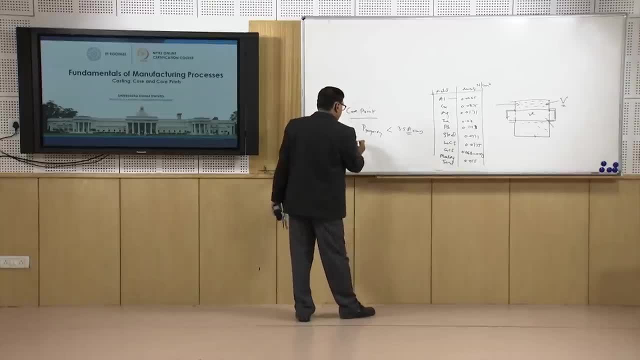 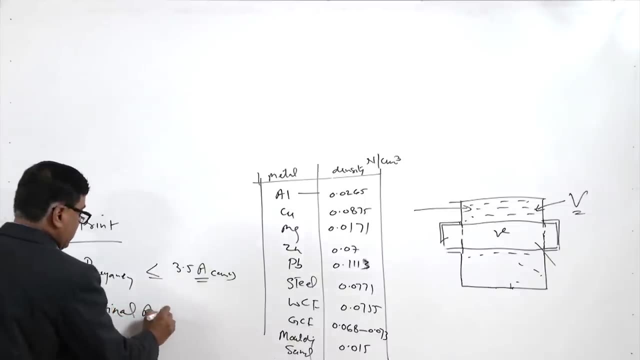 and if that is not the case, then we need to provide the additional area. if this equation is not satisfied, then additional area for support of core is provided, and for this purpose chaplets are used. So chaplets are nothing. they are the metallic pieces which are provided in the casting to 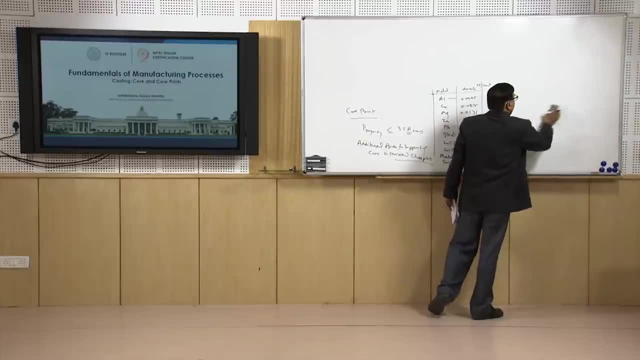 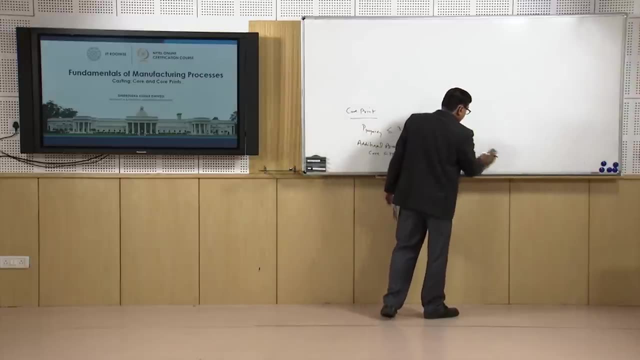 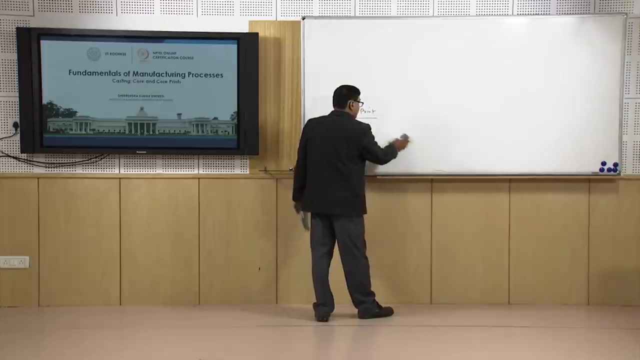 provide the support So that it can sustain the things effectively, to support the core in the mould without getting disturbed in its position. its position is maintained and it is well supported with the help of the chaplets. So chaplets are basically chaplets. 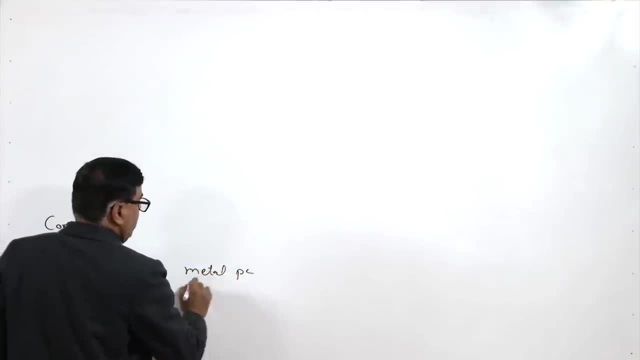 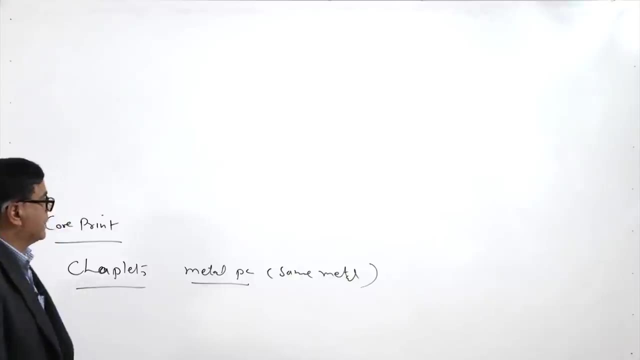 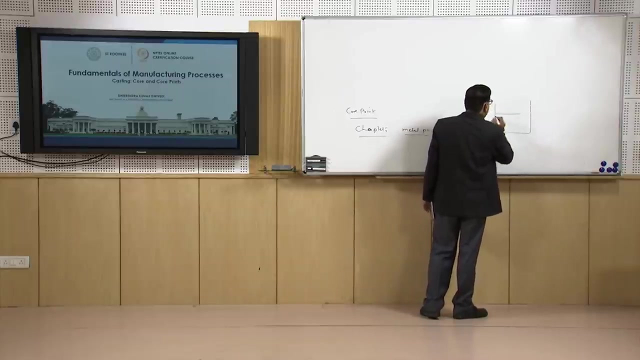 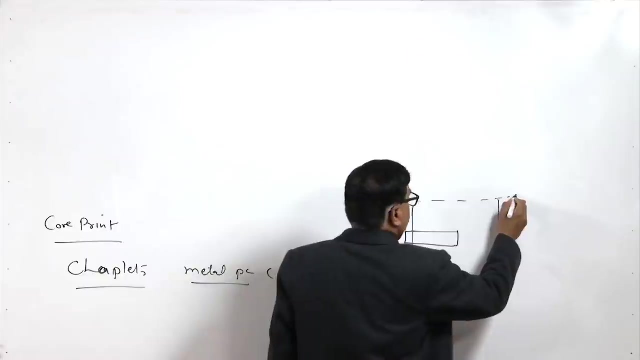 These are the metallic pieces. most of the time, same metal is used for this purpose, same as that of the casting. So if the say this is the mould and the core is positioned in this manner, it is overhanging, means. The depth of the hole here is partial and this is the core. 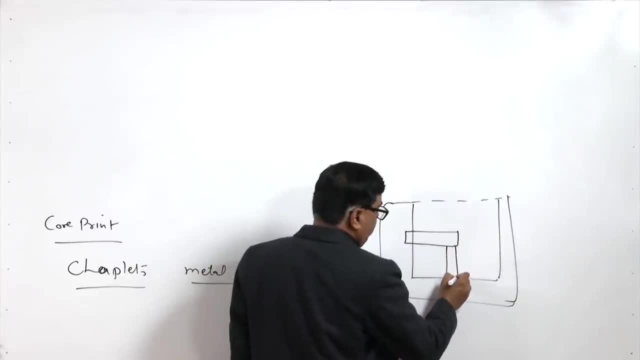 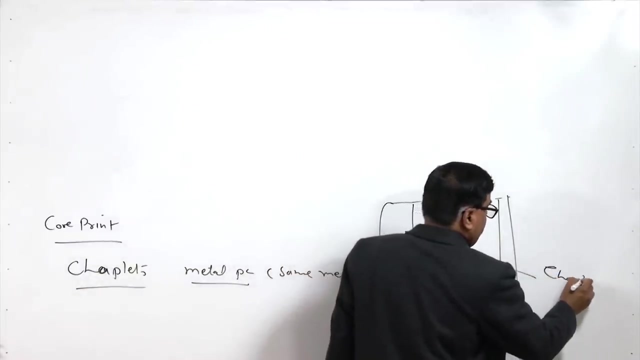 So in this case we need to provide support to the core with the help of a chaplet. So this is the metallic piece which will be used to provide the support to the core. So basically, this will be coming in contact with the molten metal. 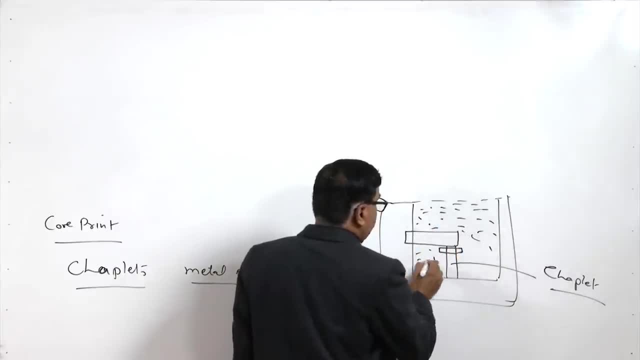 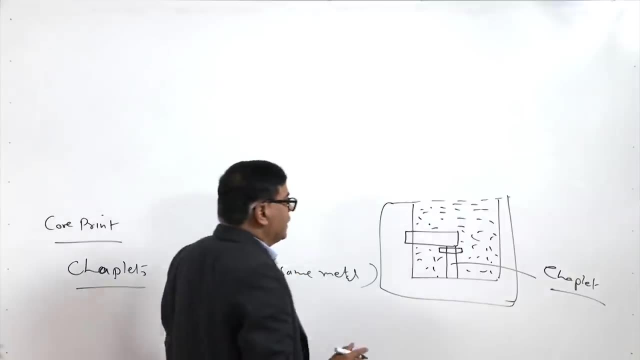 Now, what is expected From the chaplet? Since the chaplet is providing support to the core to retain its position and keep it secure in the desired position, what is desired, chaplet will be providing the support. So when the chaplet comes in contact, since it is of the same metal when it is exposed, 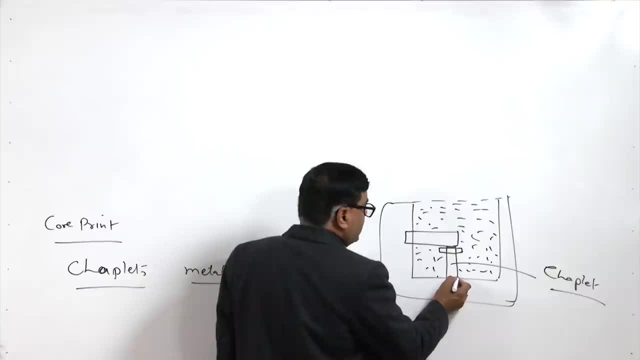 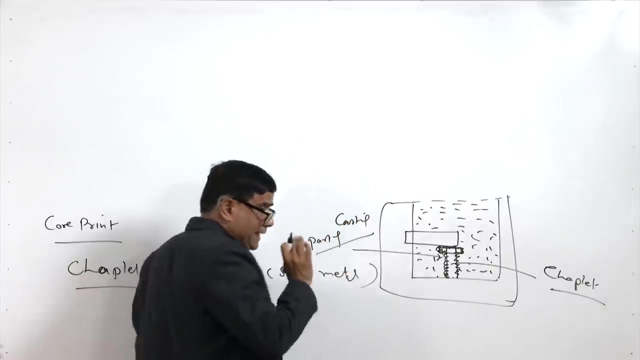 to the molten metal from all around. it is expected that surface of the chaplet will be melted and will get fused with the molten metal. So if this is the situation achieved, then it forms the part of the casting. But for this the skin of the chaplet should get fused properly, otherwise there will be 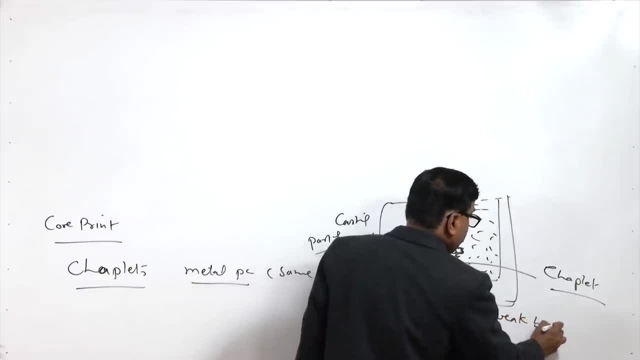 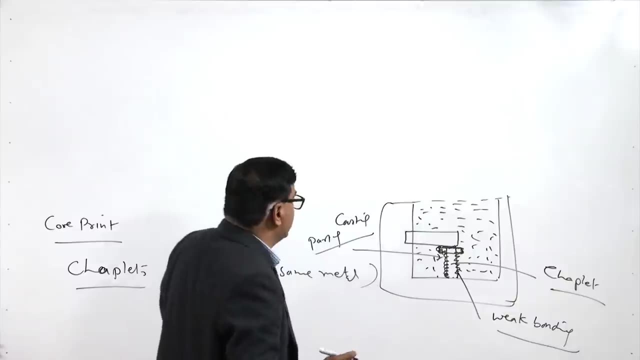 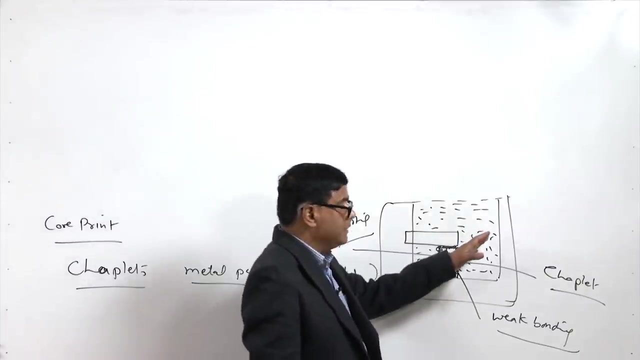 the weak bonding between the metal of the casting and the chaplet, and which will weaken the casting as a whole. Therefore. So it is desired that the size and the weight of the chaplet is selected properly, so that with the heat of the molten metal, its skin is fused and forms the proper metallurgical 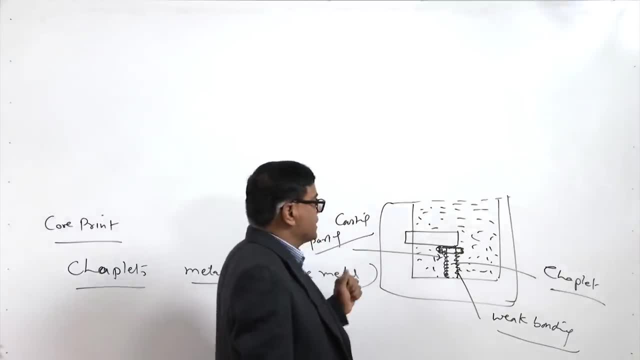 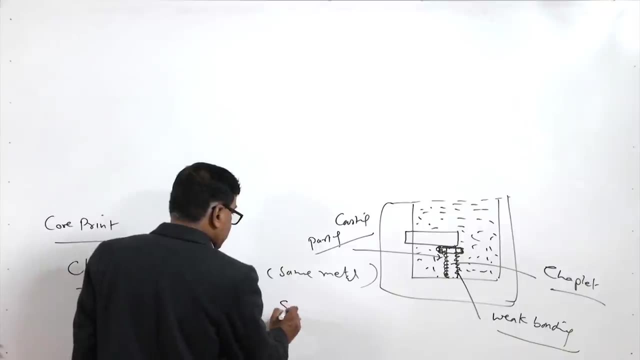 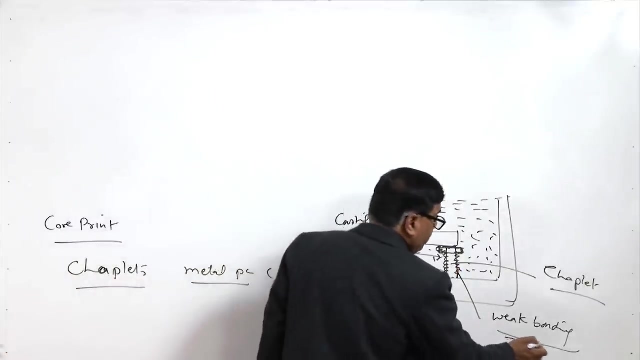 bond and it forms the part of the casting effectively. And if that is not achieved- if, like say, the size is big, then it will absorb lot of heat and still. So you may find that the bonding between the molten metal and the chaplet has not taken. 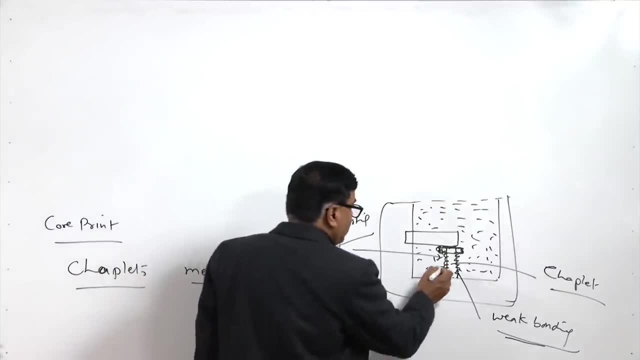 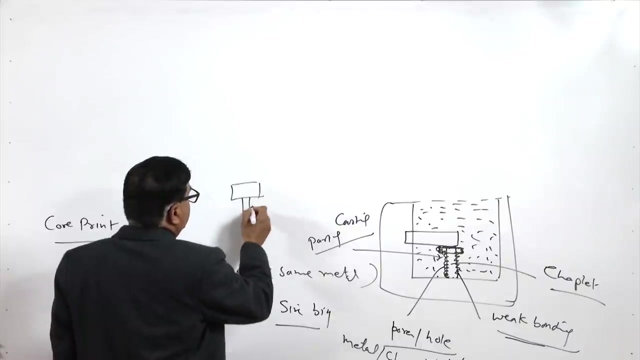 place due to the lack of melting of the skin and in that case we may find that there are like pores and the holes at the metal chaplet interface. So say, this is the chaplet And if, due to the excessive heat requirement, it has not melted, then there may be pores. 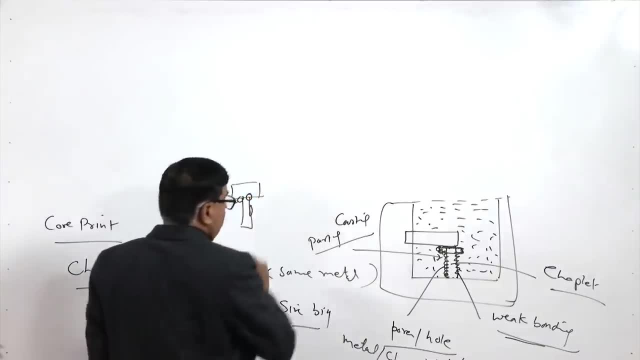 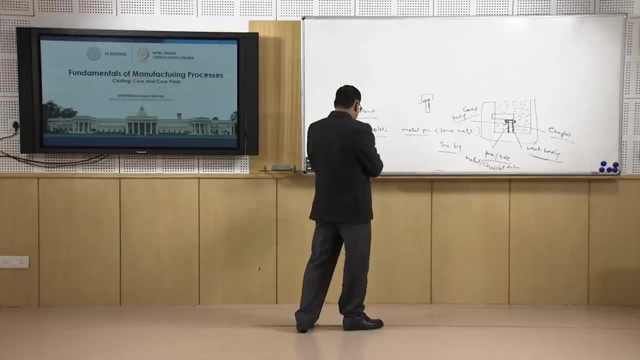 and the holes at the metal and the chaplet interface. So this situation need to be avoided. So how do we select the area of the chaplet? Area of the chaplet is selected in such a way that for that, basically, we use the same. 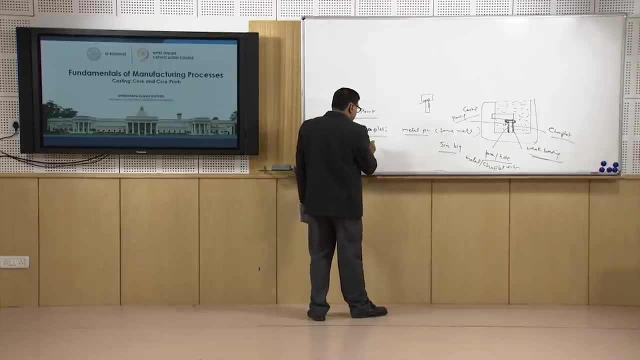 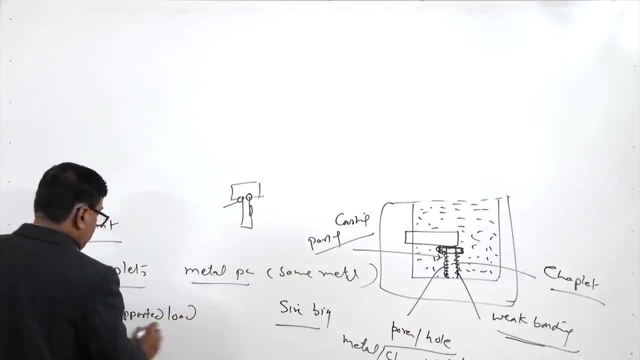 equation Like: if there is any unsupported load due to the improper size of the improper size of the chaplet. if there is any unsupported load. So for this purpose we determine one. we use one equation unsupported load if it is there in the situation when the earlier equation was not satisfied. like P is less than and. 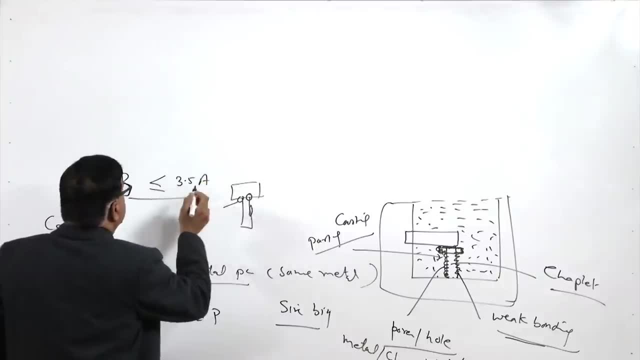 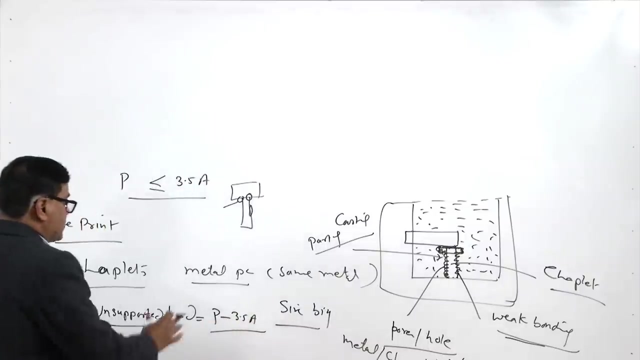 equal to 3.5 A. If this equation is not satisfied, In that case, like say, P is still bigger. So that is what that will be the value of unsupported load. and for that purpose, what we do, basically we determine 3.5 A. So this difference of this is used for determining. 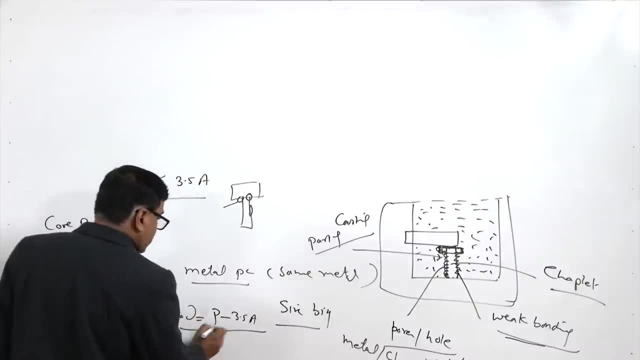 the magnitude of the unsupported load. And once this magnitude of the unsupported load is obtained, then this is what is there? unsupported load. So this is the area, So this will be in Newton, and here it is in 3.5 into A. So A here is in centimeter square. 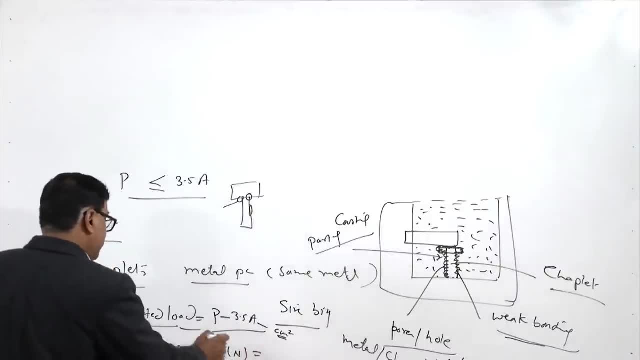 This is equal to. so we use another empirical equation: whatever value of the unsupported load has been obtained, So this will be made equal to the basically here. So this is the area, So this will be in Newton, And here it is in 3.5 into A. So A here is in centimeter square. 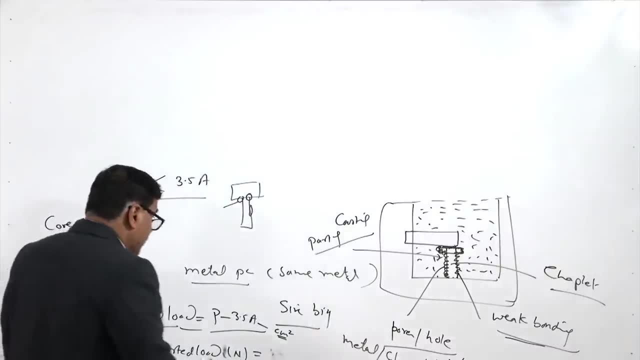 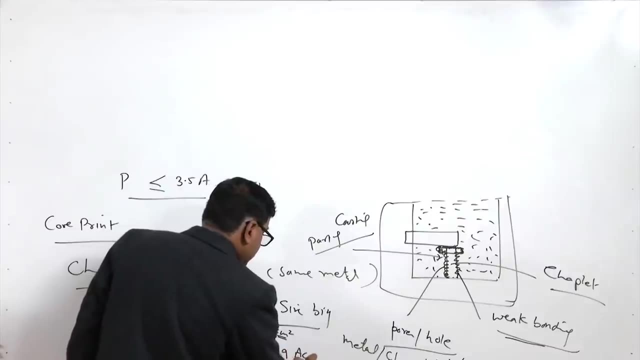 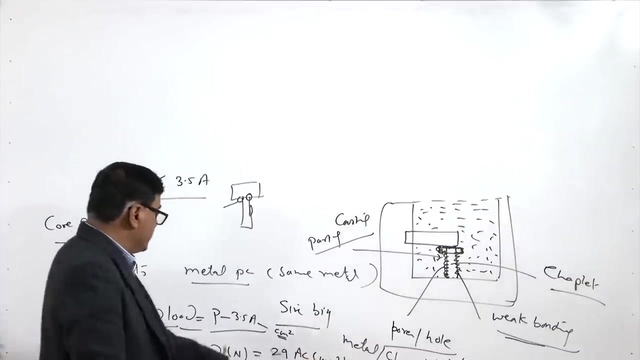 This is equal to. So here it is 29 AC. AC is the chaplet area which is desired and this is in mm square, So 29 is the like. the 29 Newton load is expected to be taken by unit area of the chaplet. 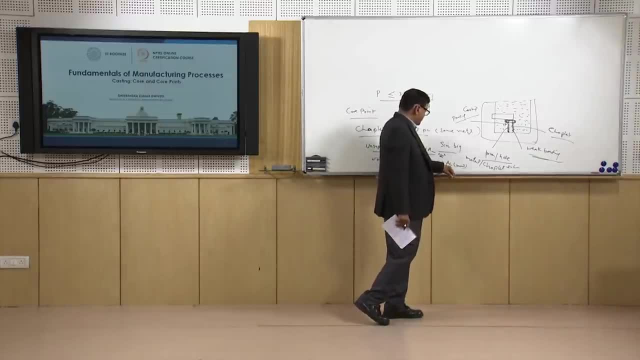 So, considering that 29 AC, AC is the area of the chaplet which is desired and it is in mm square, So unsupported load is equated with the 29 multiplied by the AC. that is the chaplet area in mm square. 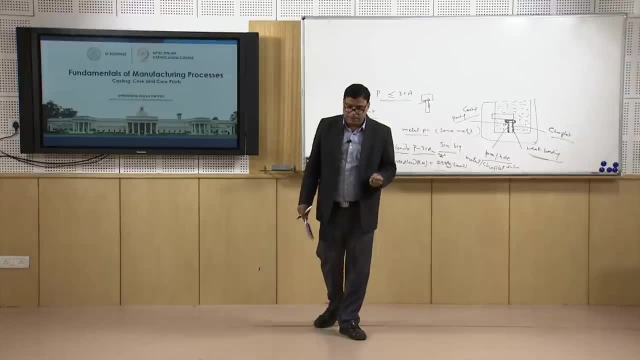 So that is how we can determine the size of the chaplet or the area of the chaplet which is to be used. So now, here I will summarize this presentation. In this presentation, I have talked about the role of the cores, different types of the 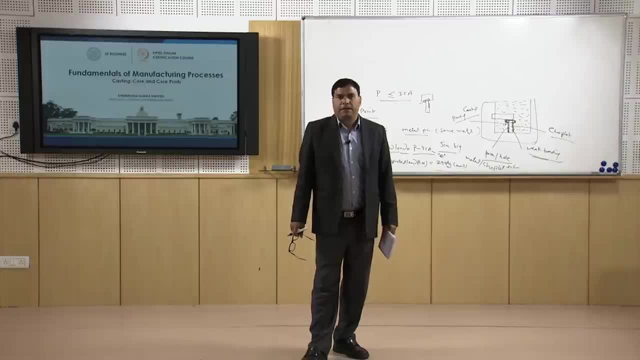 cores and how do we determine the core print size? So let us see So, let us see. So what is the core print size and what is the role of the chaplets and how the chaplet size can be determined for handling the buoyancy force effectively? 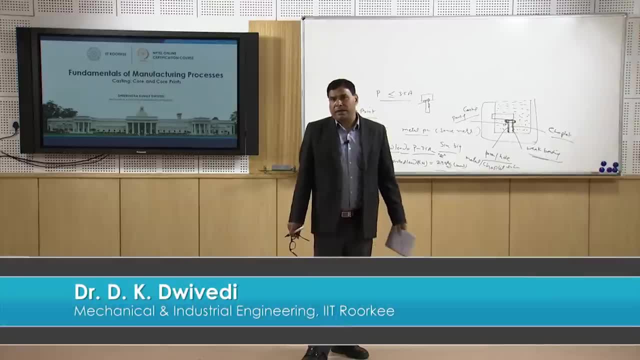 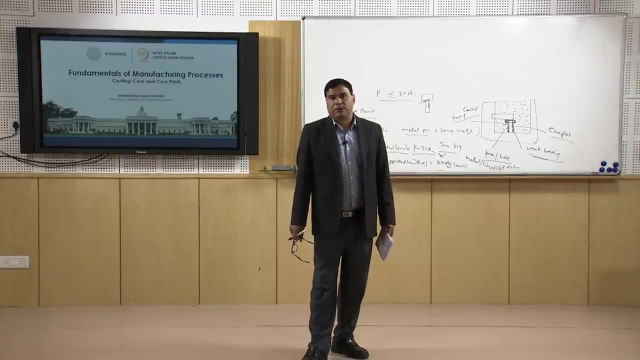 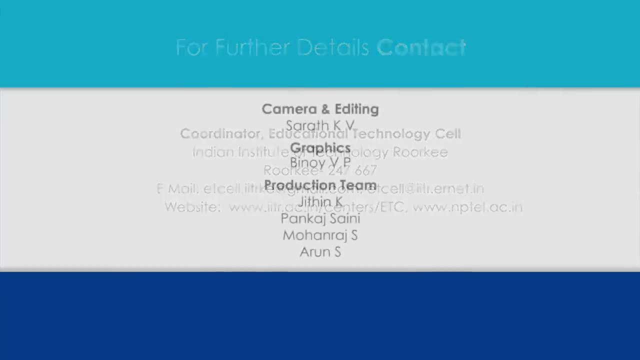 So that the core can be positioned. core can be kept in position for producing the hole and the internal features, the desired location. Thank you for your attention. Thank you very much.